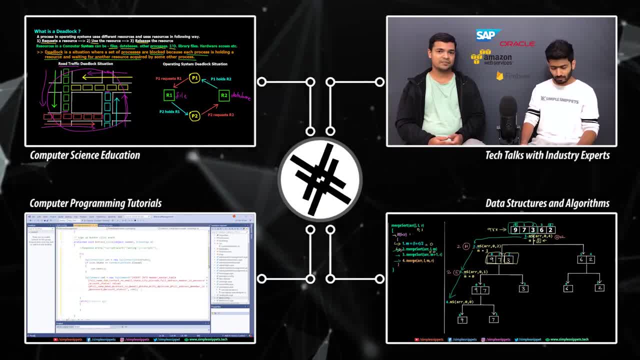 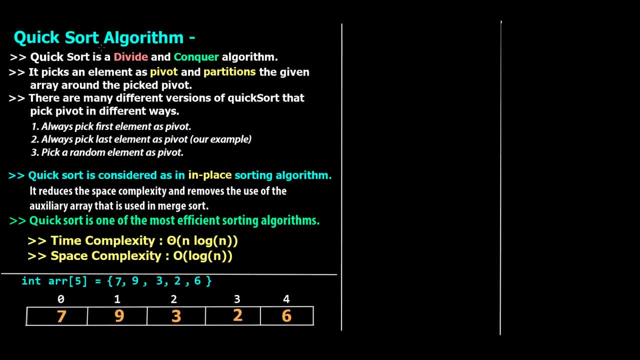 on this channel. So if that's something you're interested into, then definitely subscribe and turn on the notifications to get the latest updates and never miss out on such important topics. Okay, so quick sort sorting algorithm is a divide and conquer algorithm. Now 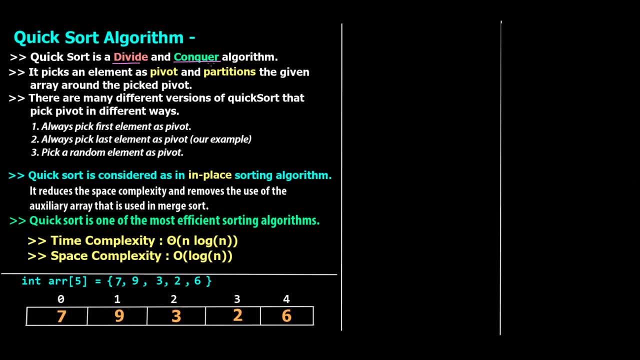 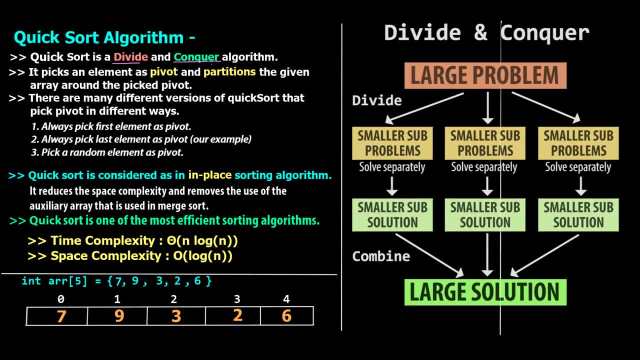 if you've watched previous tutorials. we've talked about binary search, we've talked about merge, sort, and both these other algorithms also use this divide and conquer strategy. Now, this divide and conquer is nothing but a methodology, a strategy which is used by certain algorithms, which breaks a 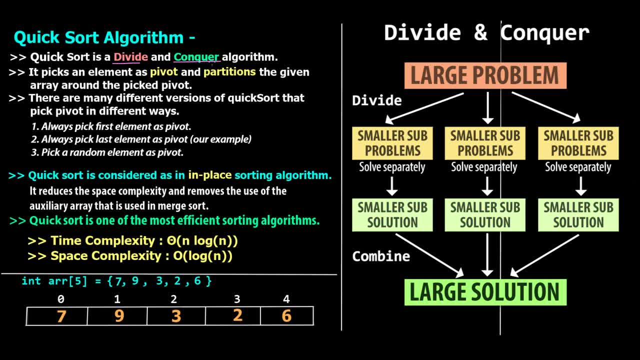 larger problem into smaller sub problems And then you solve those sub problems into sub solutions and combine the sub solutions to get the final output. Now if you're wondering why do we do this, that is because when you divide a larger problem into smaller chunks, into smaller sub problems, 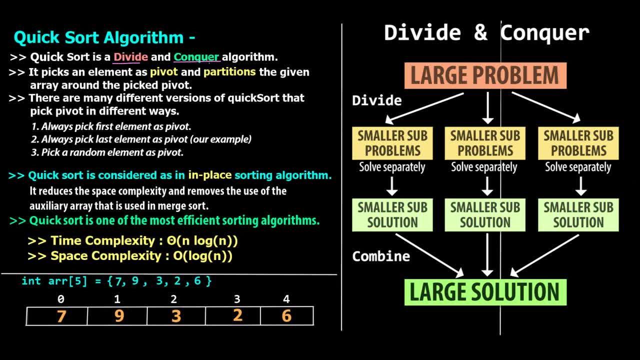 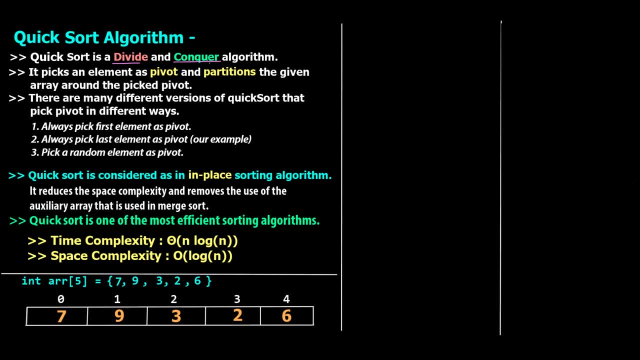 it is easier to solve those. Okay, and that's where the efficiency increases. And if you've seen in merge sort, the time and space complexity was highly efficient compared to other basic sorting algorithms like selection or insertion Or bubble sort. Okay, we've discussed all this and we've talked about time and space complexity. 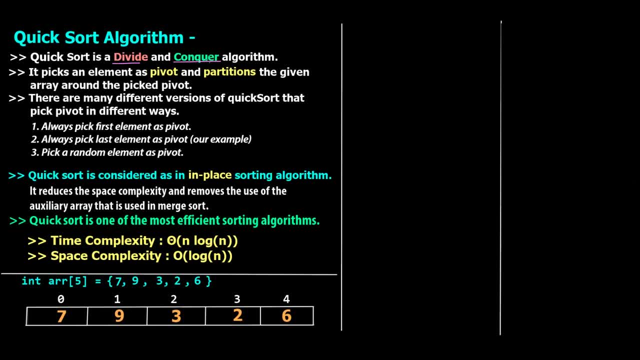 also in two separate tutorials in this course itself, So make sure you watch those. those are absolutely important. So moving forward quick sort is also recursive in nature, which means that it keeps on calling itself till a particular condition is met, So it will keep on dividing the 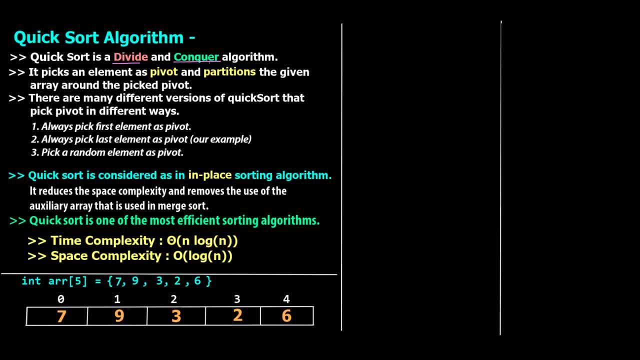 larger array or larger list into smaller chunks till a certain condition is met. In this case it would be when the entire array is divided into one element array. If it is five elements array, it will keep on dividing the array till we have only one element. 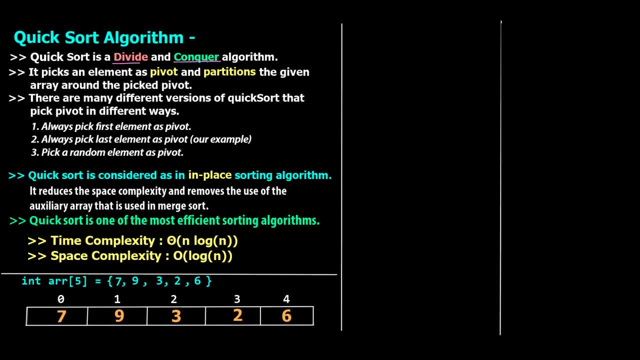 left. Okay, so that's the condition And that's what recursion is all about. It keeps on calling itself. I've also talked about recursion in other video. So this thing is similar to merge sort, but a different thing or different factor in quick sort is it uses the concept of selecting a pivot. 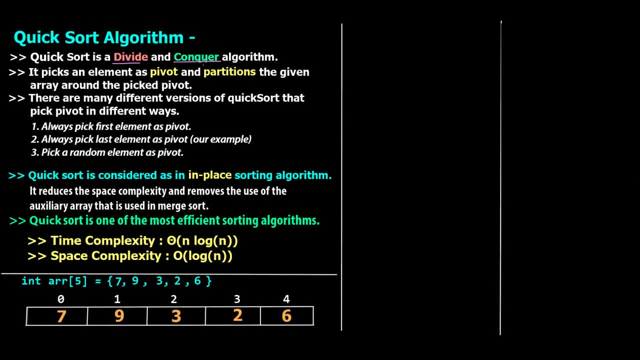 that is, selecting an element and calling it pivot. you, you know it is kind of like a midpoint. you know you can set a pivot to the center of the array in such a way that all the elements that are smaller than that pivot will come to the left and all the elements are larger than the pivot will go. 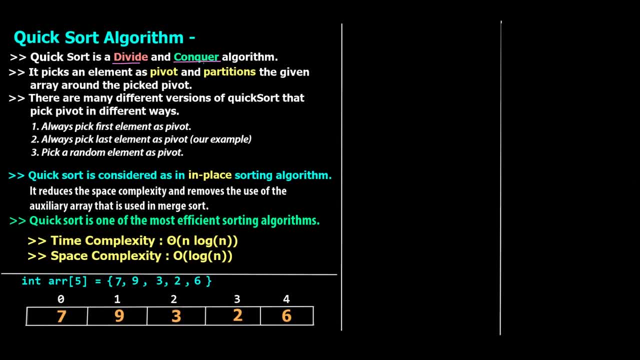 to the right, Okay, and then you apply quick sort on the left portion and the right portion. So this is the strategy. we'll talk about the working as we move ahead. And this is what point two talks about. So it picks an element as a pivot and partitions the given array around the pivot. 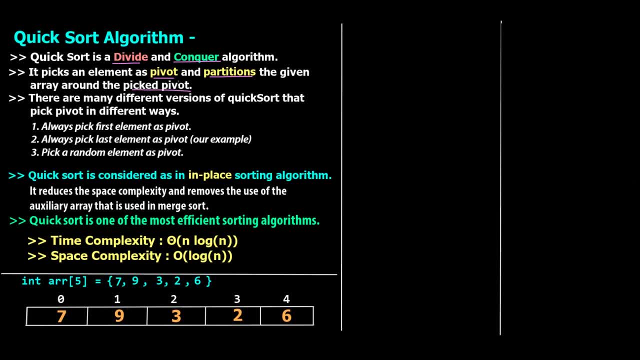 Okay, we'll talk about this point And we'll take a visual explanation also. Now, talking about the different versions, there are different versions in which quick sort can be implemented And the versions basically decide how you pick the pivot. Okay, so how you pick one particular element, as the pivot defines the different. 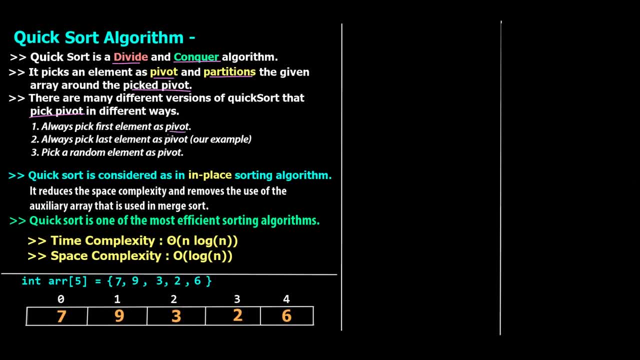 versions, For example, you can always pick the first element as the pivot. So if you pick the first element as the pivot every time for this array, for the first time this will be the pivot. Another way is always pick last element as the pivot, And this is what we are going to do. 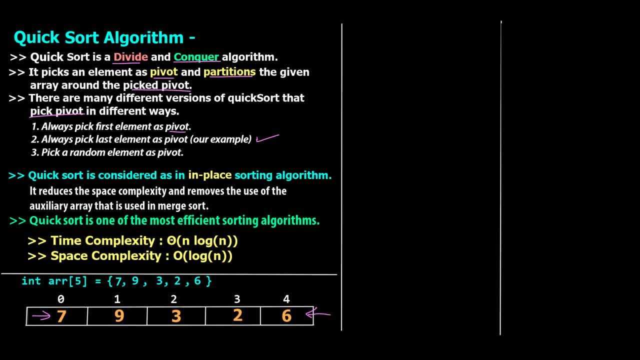 In this case, last element is this: So we pick this as the pivot, And then the third mode is: pick a random element as pivot, in which case you can randomly pick any of the element as the pivot. Okay, so these are different ways or different modes in which quick sort can be implemented. 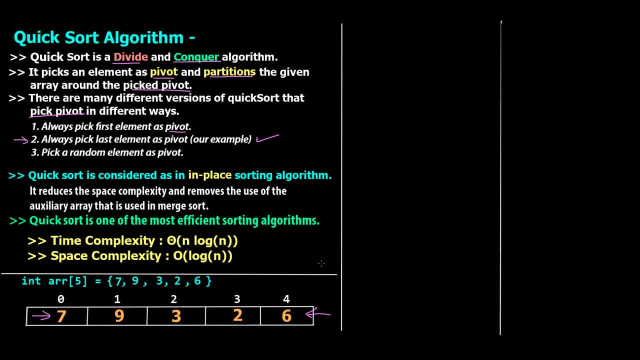 We are going to implement the second way, which is always pick the last element as the pivot. Okay, Now another differentiating factor between quick sort and merge sort is quick sort is considered as an in place sorting algorithm. So just like selection sort, just like. 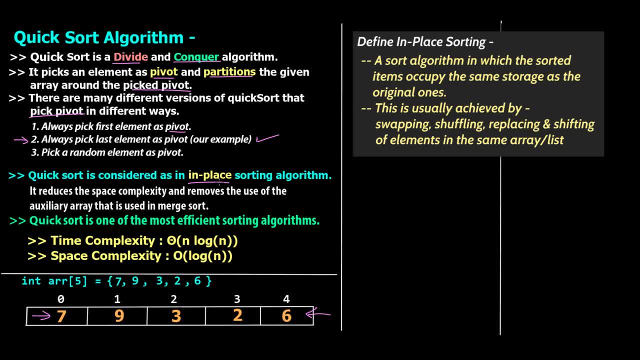 insertion sort, just like bubble sort in place sorting algorithm sorts the existing array in its place itself, which means that it uses swapping, or you know, substituting or replacing of elements in the same array. It does not require a separate array or temporary memory to perform the sorting. 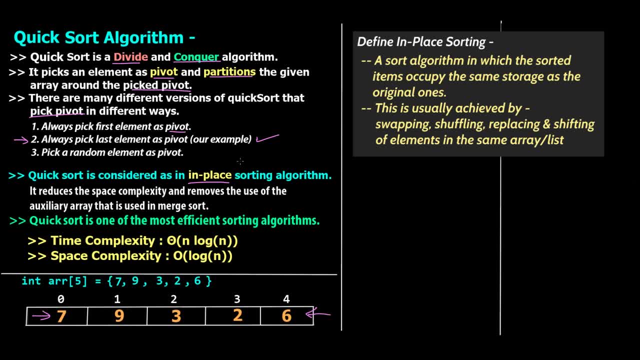 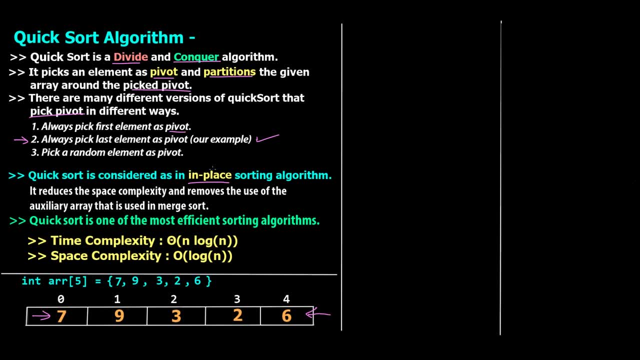 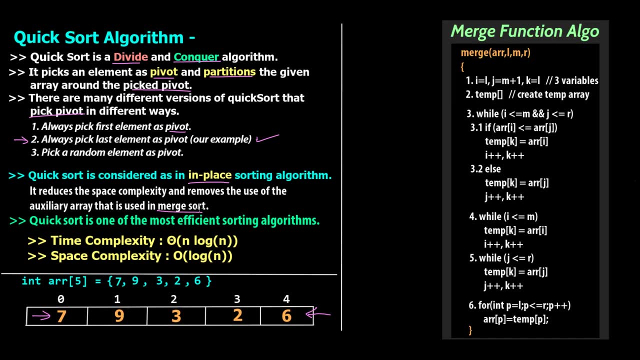 So this is what in place sorting algorithms do: They sort the array or sort the list or data structure in that place itself and you do not require extra memory to sort it. So this reduces the space complexity and removes the use of auxiliary array that is used in merge sort. So, if you remember, in merge sort, in the merge function. 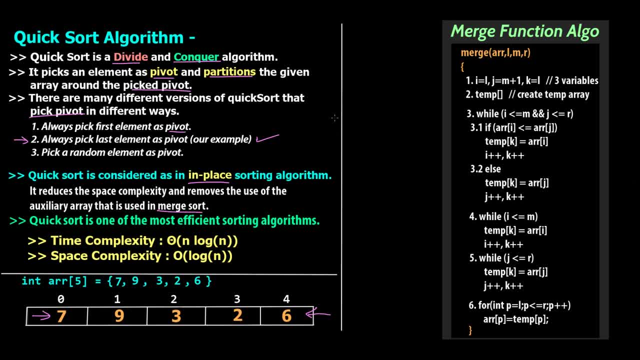 every time we were merging back the sorted sub array, we were using a temporary array right. So that is called auxiliary space or auxiliary memory, which is just nothing but extra space. We've talked about space complexity and this in this merge sort, since at every merge step, 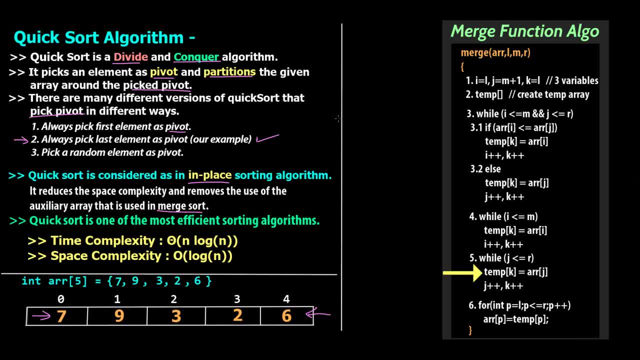 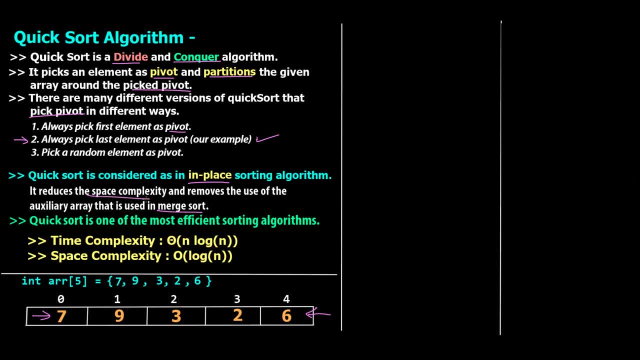 we have to create this temporary array. some extra memory is utilized, right? So that is not required in merge sort, And hence quicksort is considered to be more space efficient compared to merge sort. So hence quicksort is also one of the most efficient sorting algorithms. And, if you observe, 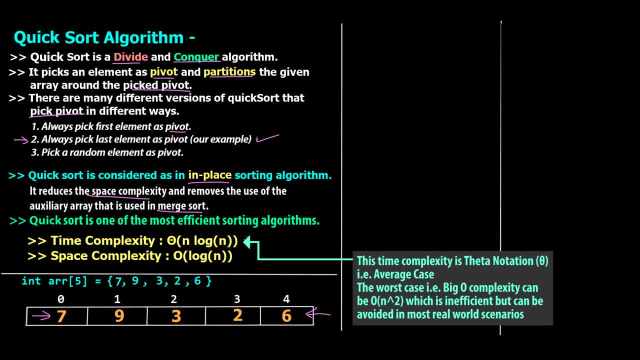 the time, complexity is n, log n, which is pretty much similar to merge sort. However, the space complexity is O of log n. In merge sort, the space complexity was n and log n is kind of less than n on the graph if you plot it, And hence quicksort is a little bit more efficient when it comes to. space complexity. So this was it for this video. If you liked this video, please subscribe to my channel and hit the bell icon so that you don't miss any of my future videos, And I will see you in the next one. Bye. 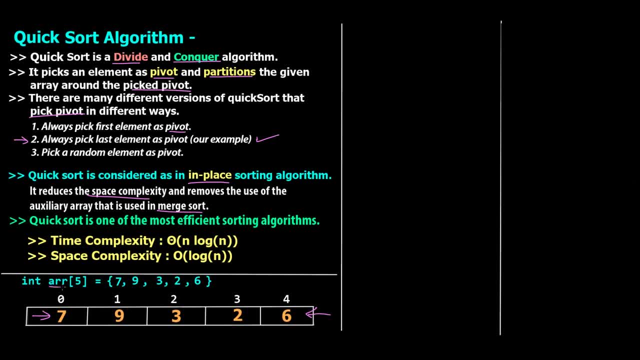 little bit of theory, And this is the array that we're going to use in our example. it is going to be an array of size five and having elements seven, nine, three, two, six, And talking about this point, that is, you know, the second point- it picks an element as a pivot. 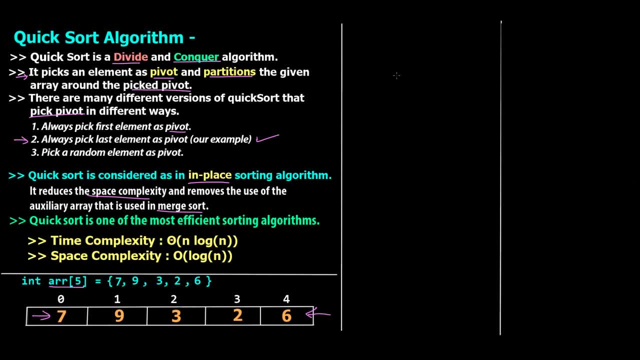 and partitions, the given array around the pivot. So just to give you a visual representation, let's say we have this array And this is our array, right: Seven, nine, three, two, six. Now we're going to use this mode, that is, always select the last element as pivot. So in step number one, 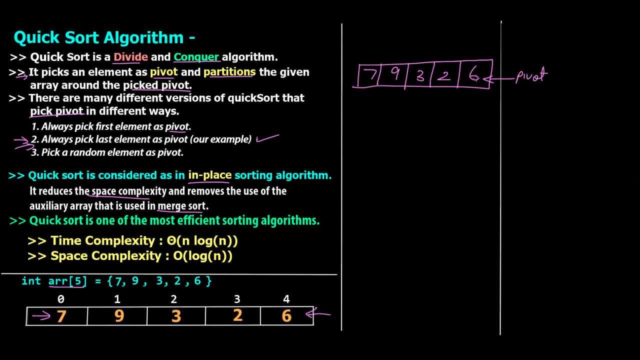 in first quicksort. we're going to select this as pivot And what we will do is, after this one step of quicksort, this six will be positioned in this array in such a way that all the elements that are larger than six will come to the right hand side of the six and all the elements that are smaller 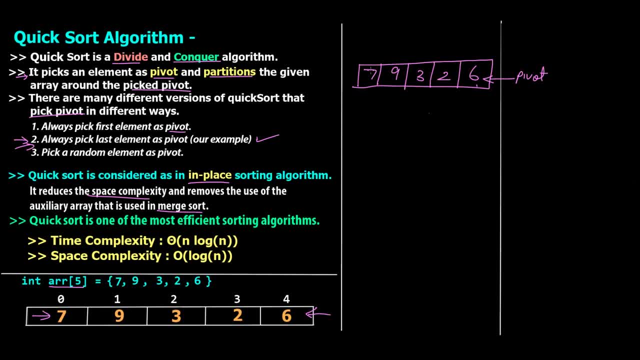 than six will come to the left side. So let's see which is larger. So if seven is larger than six, seven will be placed over here. nine is larger than six. nine will be placed over here. six will come in the center. three is smaller than six. three will come over. 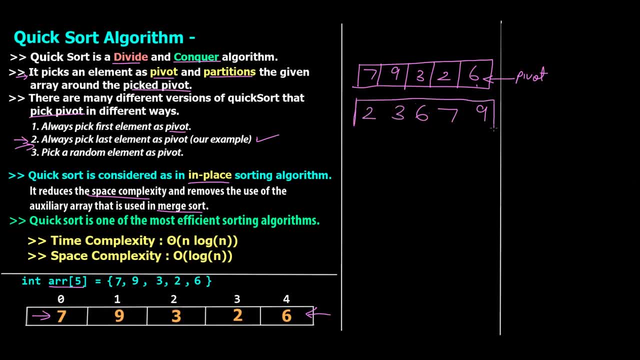 your two is smaller than six, two will come over here, And this is after step number one. Okay, so we have multiple recursive steps And right now the array is not sorted. Obviously, it is not sorted in one step, But, if you observe, what has happened is six has come in the right. 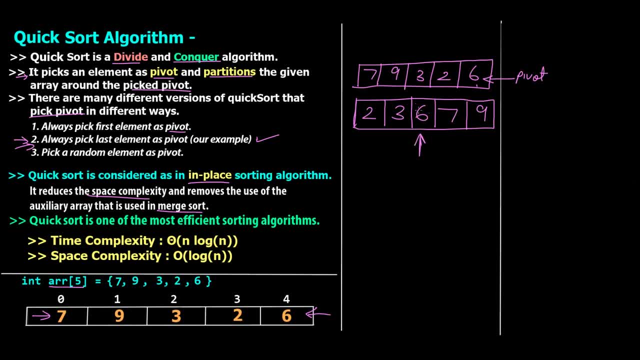 position in the center position where it should be. So now this pivot, that was six value- has come in the center position after one step. Now, if you observe, two and three on the left hand side are kind of sorted, and seven and nine is also sorted. But this may not be the 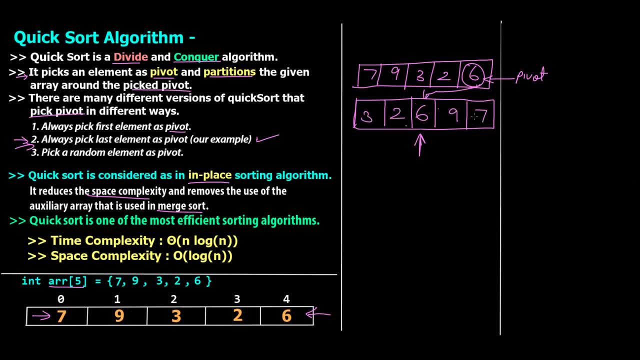 case you know, it can also be three 297, something like this. I was just showing it for representation purpose. But after step one, what will happen is the selected value. the pivot will come in such a position where on the left hand side of the pivot will be all the elements. 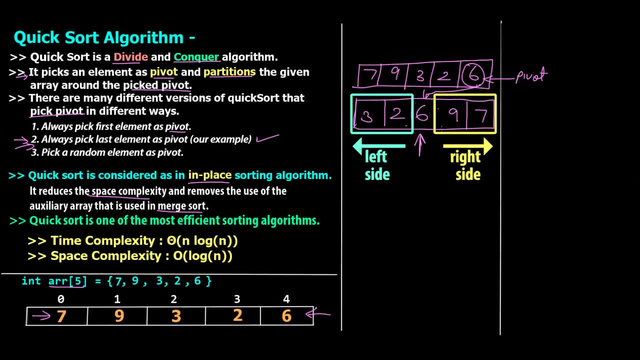 that are smaller than that pivot value. And on the right hand side of the pivot all the values will be greater than the pivot value. So this is still not sorted. But now what we will do is we will apply quick sort again on this sub array and this: 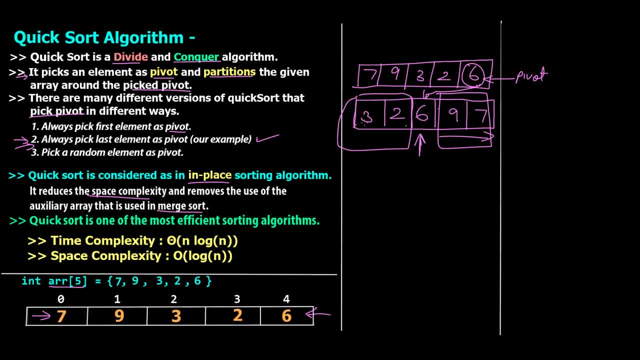 array because six has come in the right position, right. so now we have to apply quicksort over here for these two elements and these two elements, so two more quicksort calls and so on. it will progress till the entire array is sorted. ok, so i hope you are getting a little. 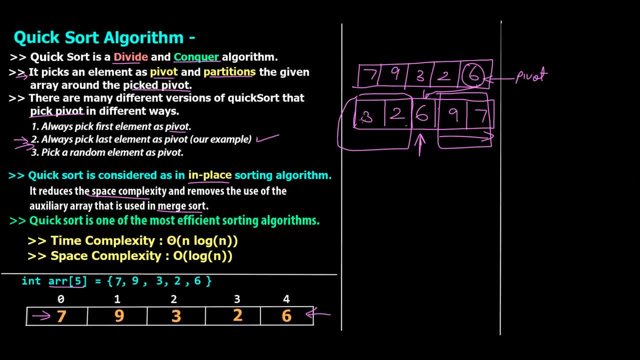 bit of the working. of course, we still have to see the algorithm and we will dry run this algorithm also, but i just wanted to give you an overview about how this pivot is selected and brought to a position where all the elements to the left are smaller than that value and 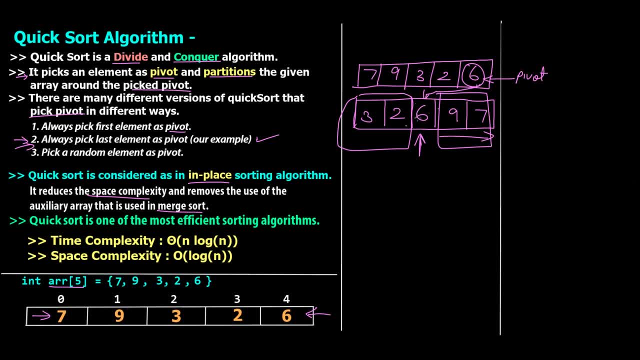 all the elements to the right are larger than that pivot value. so this is the entire concept at the overview level. now what we will do is let's take a look at the steps that are involved in the quicksort sorting algorithm. so, at the overview level, in a you know step, 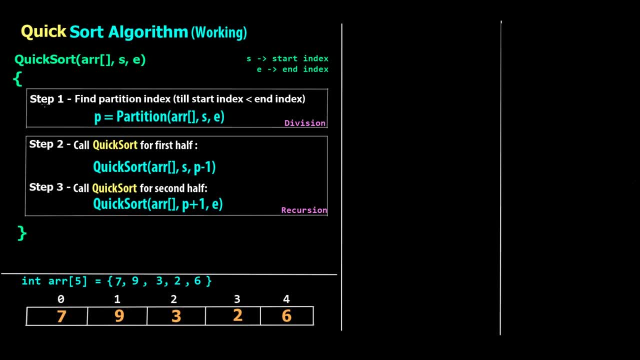 by step representation or you can see this is kind of like a english version of the algorithm. we have the function name quicksort, we have the array arr that is passed s and e represents the start index and end index. so there are three major steps and you know two parts. basically, if you've seen the merge sort, there was a fourth or 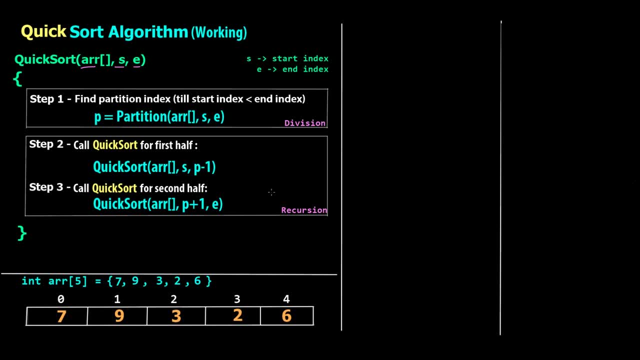 third part, which was merging. but over here we don't need to merge it. so step number one is find the partition index. so we need to find where exactly are we supposed to partition every time, right. so that partition index is supposed to be found out, and this is where 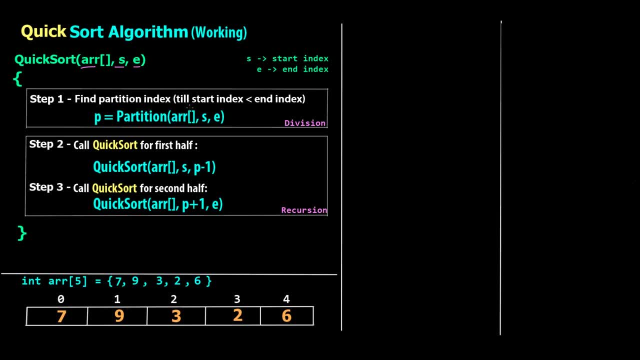 the recursion will happen because this partition will keep on happening till the start index is less than end index. obviously, start index will be less than end index every time till we have only one element in the subarray. right when we have only one element in the subarray, either the start index and end index will be equal or 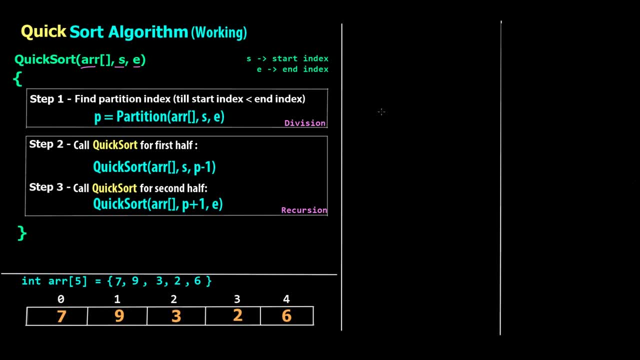 the end index will go below start index. so you'll see that in the working, don't worry. but this is where recursion will happen and we will keep on calculating the index where we are supposed to partition or or find the pivot value. okay, now, this partition is a separate. 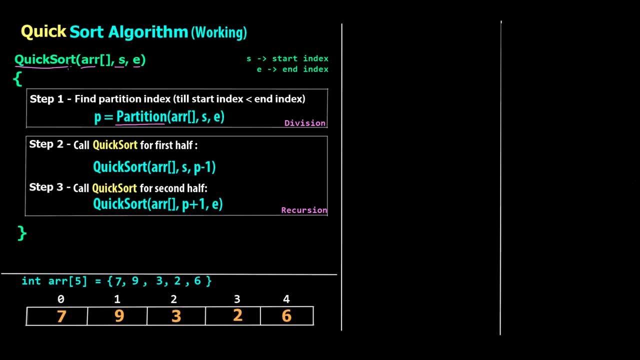 function which is called inside quicksort. so quicksort is a function- or you can say method- inside that we are creating another partition function which will take that same array and same start index and end index. and here is where the division is going to happen. division is where we are finding the pivot point or partition point to be divided into. 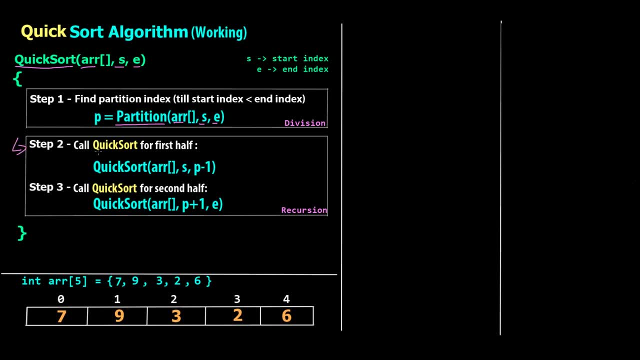 two subarrays. now moving on to, step two is where we call quicksort for the first half and step three is called quicksort for the second half. now we just found out p, which is the partition point. then we will say quicksort of array. we will say start index as s only. 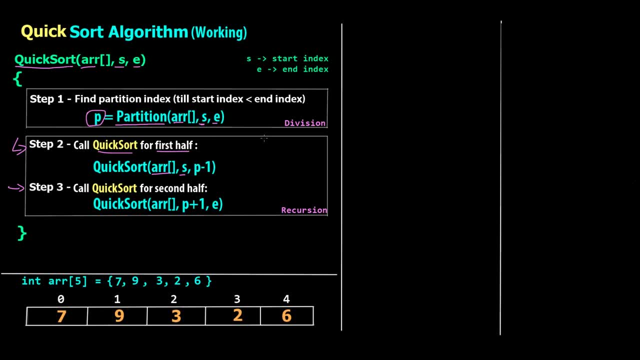 but now the end index, we will pass as p minus one because we just found out the pivot point right. so again, taking the example of phi element array, with the same example: seven, nine, three, two, six. so after first time we were having six, in the middle we were having three, two. 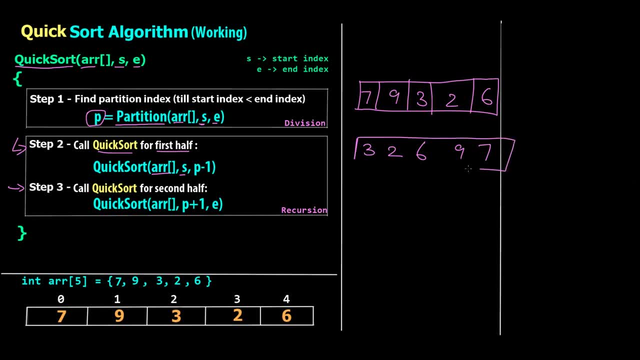 nine, seven, something like this. this is just for representation. and now, when we are calculating p, we will get something like this point right. so when we say quicksort of error of s, we will say s is going to be zero, and this is zero: one, two, three and four. and this time 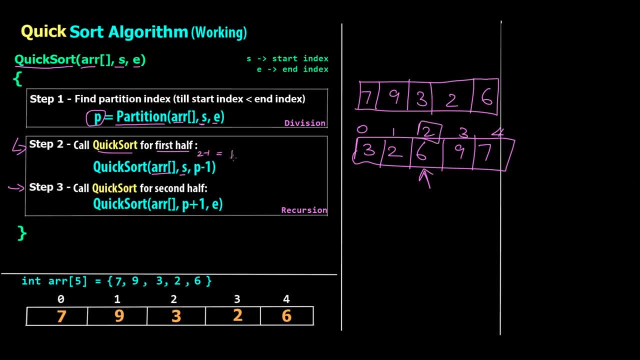 p, we will get us two. so two minus one will equal to one. so we will run quicksort, that is, this quicksort for zero to one. and the step number three is saying quicksort for the second half, which is this half. so it would be p plus one, that is, two plus one. that is: 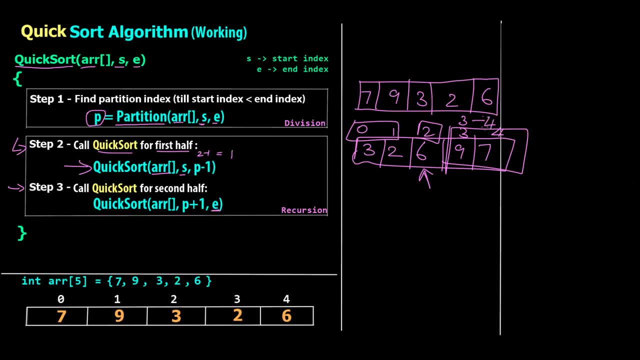 three, two and index, which is four. okay, so we will again call quicksort recursively. so quicksort is this function and we are calling quicksort again. so this is a recursive call and over here is also a recursive call, kind of like what we were doing in merge sort, but this time it is on the two. 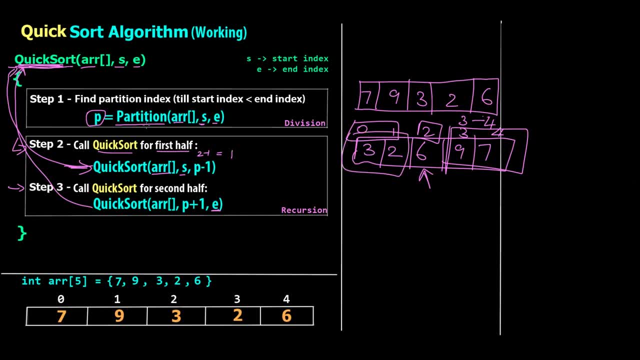 separate sub arrays and the sorting part is happening in the partition function itself. so if you are wondering where exactly is the sorting also happening, it is happening inside this partition function. so the entire crux of this entire code is inside the partition function and not in the quicksort function. okay, so quicksort function is just used to. 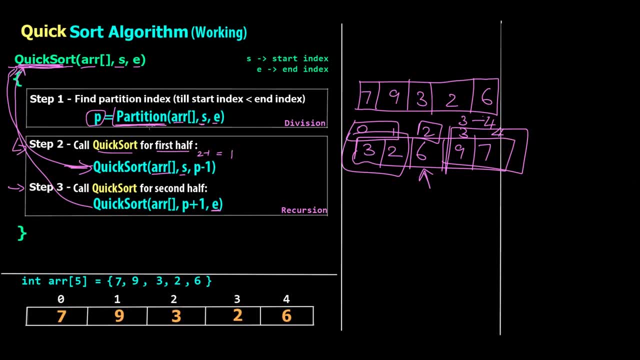 give recursive calls to do the partitioning and to do the in place sorting. so this was just a overview way. if you want to note these steps down, if you want to prepare your exam answers, you can completely note these steps down. and now what we will do is we will move to the actual algorithm. 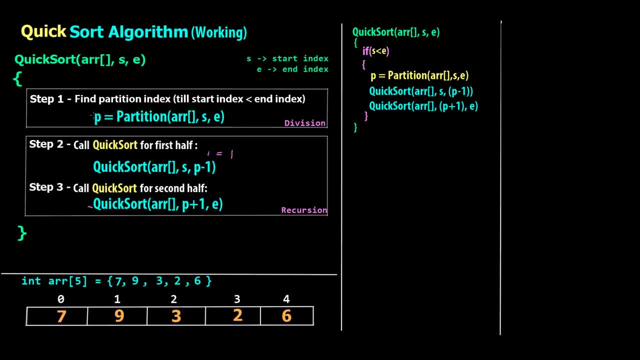 okay, okay. so on the right hand side, as you can see, i have converted these three steps into a function way, into a algorithmic way. this is still not proper syntax, okay, so this is not c plus plus syntax, even though it does look like it, it is still not proper code. so 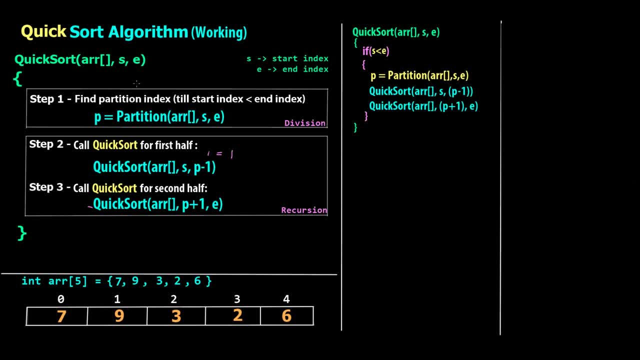 this e, which will vec, must be in the information. so we will do the simple abstraction according to the rule. it was a проц needs a such thing by ourselves to complete the record, or else the error on your computer Front grande is, if we eat the operation method, that first. 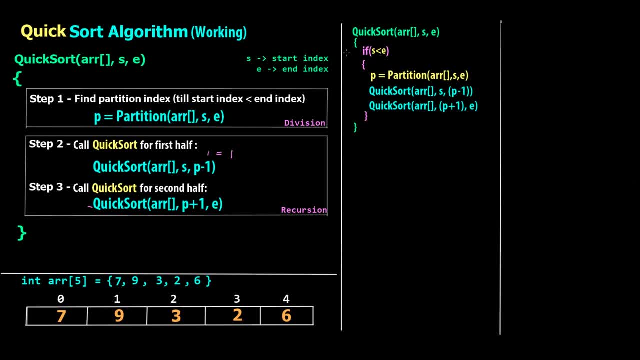 we just leave a variable state as stalling type. second, we will work it out using a small fraction struct system like log. right here. let us call this sentence like log and you will see that we don't need to use the extra number, because we don't need. 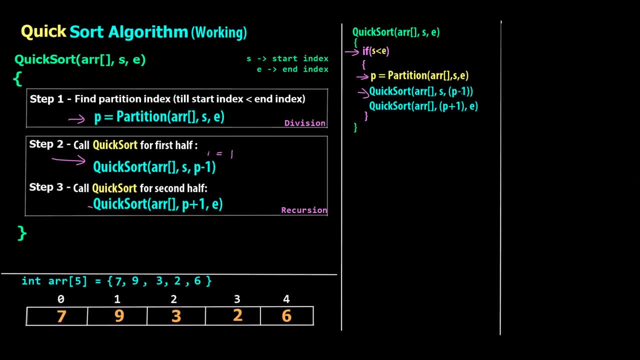 to use only the initial number and just. namely, we are giving some distance to the ends and affecting the iteration and leaving the last one empty. and we have this right in our code, which is our integration. by the way, getting the也. by the way, getting the extension by the end, start in the first and the final, Forget the. 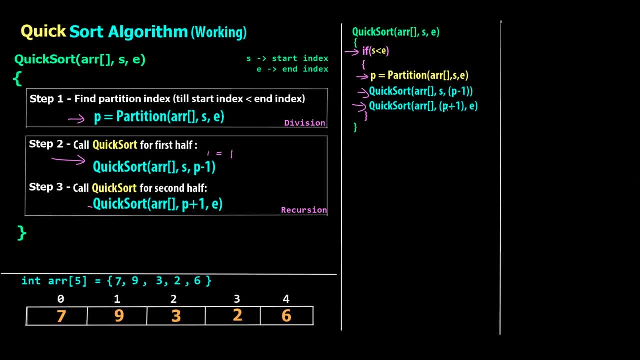 for the second half. okay, or the second partition, which is p plus 1 comma e. Simple enough. this is the quick sort function representation, but the real game or real working is actually happening in the partition function. So now let's see how the partition function progresses. okay, because 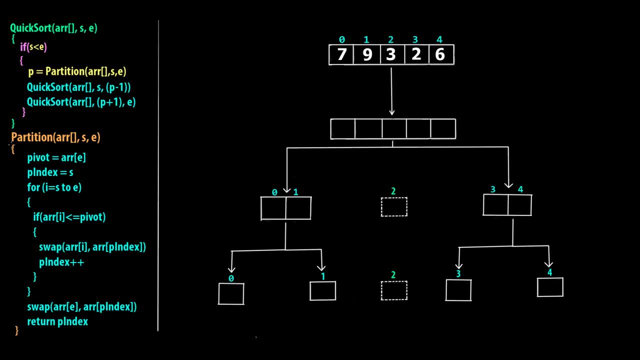 this is very important. Okay, so, as you can see, on the left hand side, I have shown you the partition function, or partition algorithm. These are the steps, different steps, that are going to happen in the algorithm, and on the right hand side, I have drawn a basic diagram of how the algorithm is. 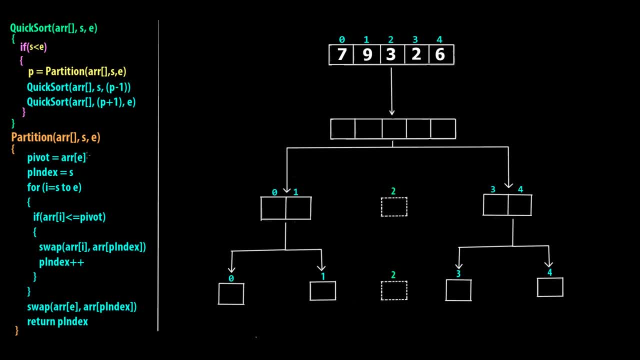 going to progress. So the best way to understand this quick sort sorting is to dry run this entire algorithm. okay, So we will go step by step, right, So we will understand what is happening at every step in the partition function also, and the best way, as I mentioned, is to implement these two. 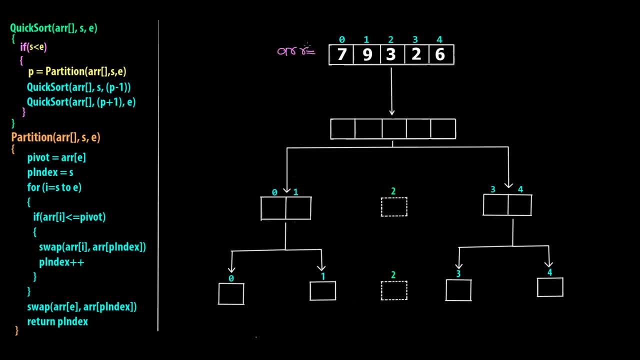 functions onto this array. So this is our array and now we are applying quick sort on this. okay, So let's start with step number one. So step number one obviously first call quick sort. So let's see how that call would look like. Okay, so the first quick sort call has happened. okay, because it is a recursive. 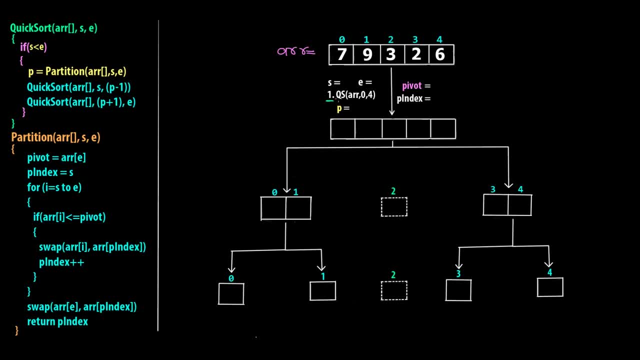 function. we will have multiple quick sort calls, So I have denoted it by number one and qs stands for quick sort. We are passing the array arr. okay, I have not used brackets, but understand that this is just representation and the start index, obviously for the first time, is going to be zero. 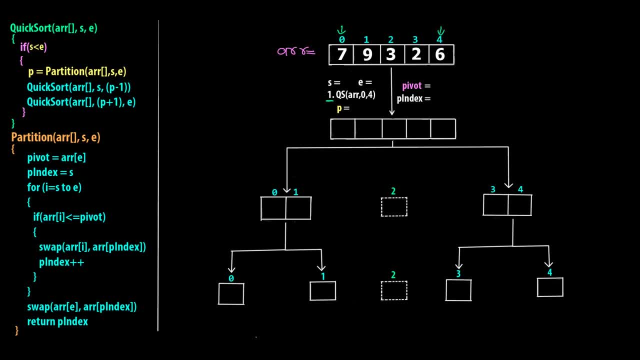 and index is going to be four, right. So when we call the quick sort function for the first time, it is going to be zero and index is going to be four, right. So when we call, the first step is: if s is less than e. Now what is s over here? Zero, right, We are passing zero over. 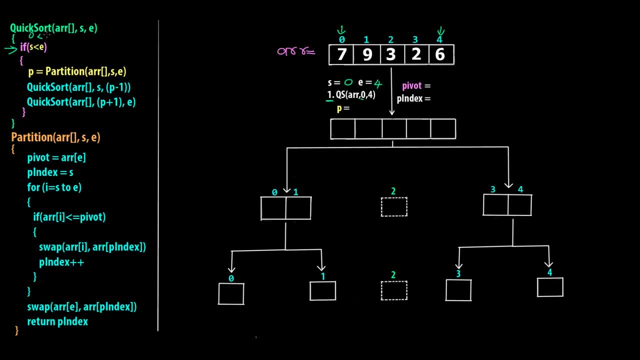 here. What is e? Four Is zero less than four. Yes, So this condition is true. We will go inside the if block. First step itself is get the partition index p, and for here we are calling another function named partition. We are passing the same array with the same s and e. okay, because 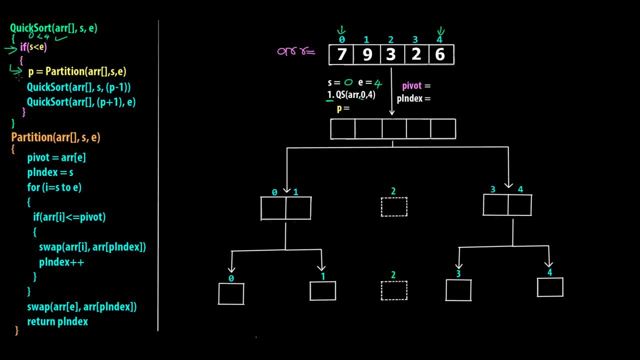 s is zero, e is four. Now, from here we will just call the partition index p, and for here we are going to jump to this partition function. So this is where the real game is happening. Real crux is happening, right. So now let's try to go step by step with the partition function. 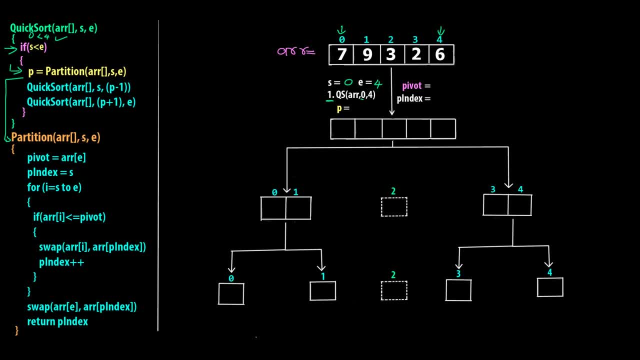 We are passing the same array, arr. We are passing start index as zero. We are passing end index as four. Now, according to our mode of implementing quick sort, remember we were saying the pivot that we are going to select is always going to be the end value of the array, or subarray, In this case, arr of. 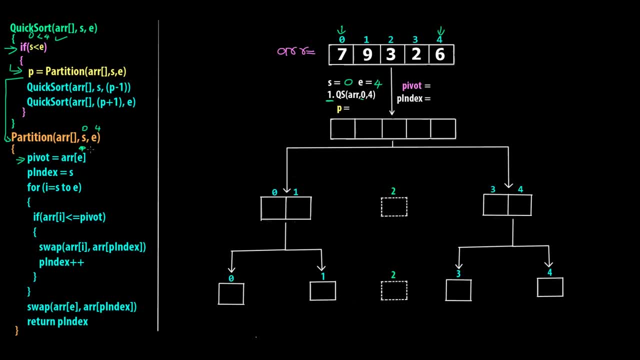 e is arr of four, because e is four, right, We've passed e as four. So arr of four is going to be what? Six? So, for the first time, this is going to be our pivot value. okay, So pivot, I'm going to. 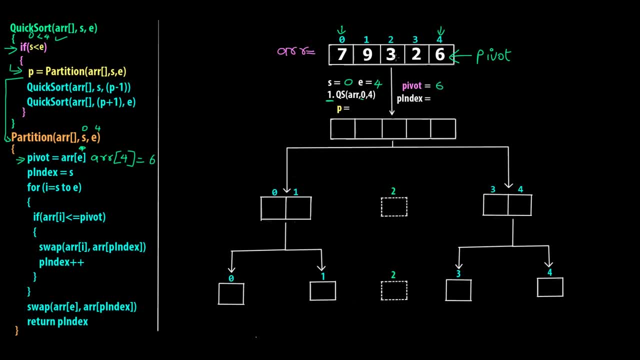 write over here is six. So every time we are going step by step in a dry run scenario, always note all the variable values so that you understand what is happening at every step. So what you can do is you can take a pen and paper yourself and dry run along with me. 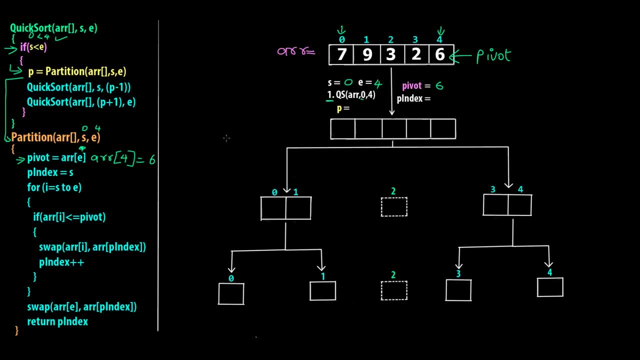 Don't take a pen. take a pencil, because you'll have to probably erase a lot of things. but that's the best way to understand such algorithms: by dry running them on pen and paper or whatever you have, and then you'll understand it in a much better way. Okay, so moving ahead. the next thing is we create another. 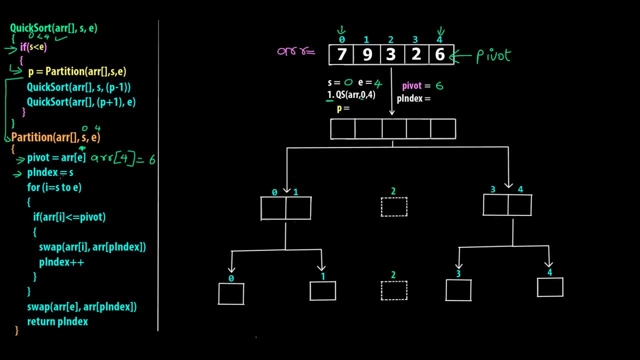 variable and we say p index is equal to s, So s over here is zero, right? So p index obviously initially is going to be zero. So this p index, I'll tell you why we're using it, but in the overview, what I've told you is: 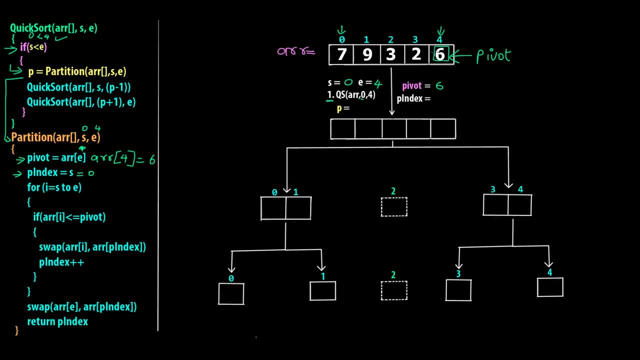 when we select one pivot, what we want to do is all the elements that are smaller than the pivot have to come to the left hand side of the pivot value, and all the elements that are larger than the pivot value have to come to the right hand side. So that is something that we have to do in this. 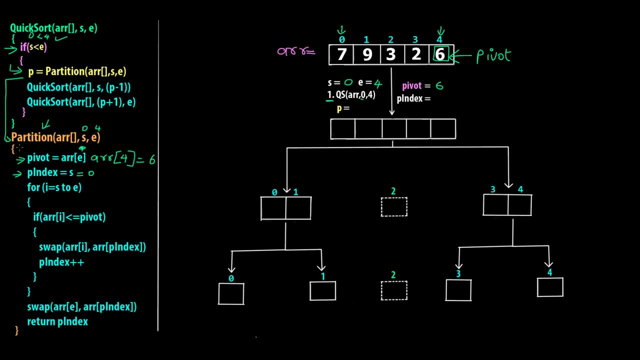 function itself. That's what I've told you. So we have to do the comparison in this partition function only. So this is where the comparison will now start right, because we want to compare every element with this pivot value individually. So, for example, if I choose the pivot value, the pivot value will go to zero. 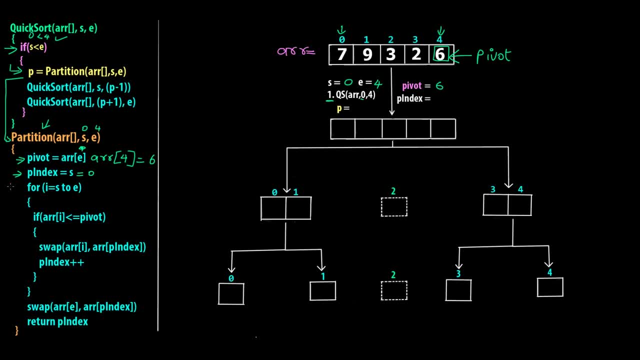 but then what I'll do is we'll select this pivot, Thomas, shouldn't I want to specify here the pivot value, I'll choose something that's smaller. Okay, for this method. we'll do this tag p index and say that p are two Naomi's for the compiled p index, and I'll 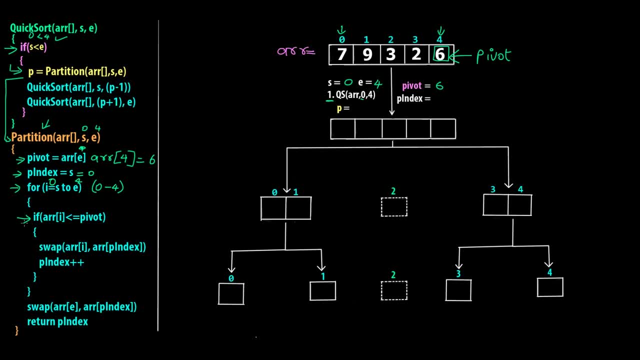 doing this with this p index on. so, for example, this position, which is currently zero, then if we want inside this, this is where the comparison is happening. So now I'm seeing if ARR of I is less than or equal to the pivot value. If it is less than or equal to the pivot value. 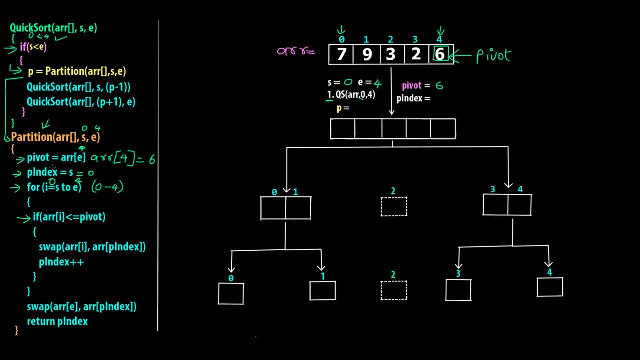 what we're doing is we're seeing swap ARR of I and ARR of P index. So let's understand this with step by step explanation and I'll tell you what is happening. So, for the first time, ARR of I is ARR of zero. What is ARR of zero? ARR of zero is seven. So we're seeing 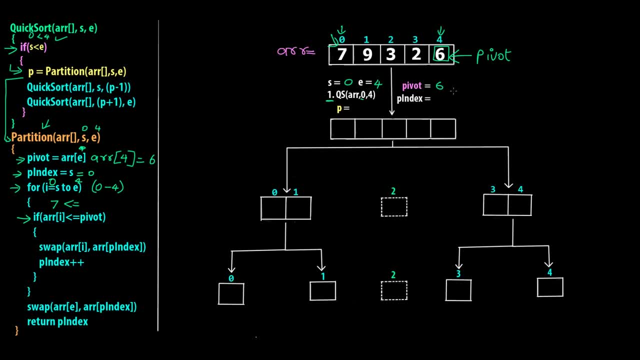 if seven is less than equal to what is pivot value. Pivot value you've decided as six Is seven less than equal to six. No, So this entire if block will not be executed for the first time. right? So it's not executed. Now we'll come at the end of the if block. we 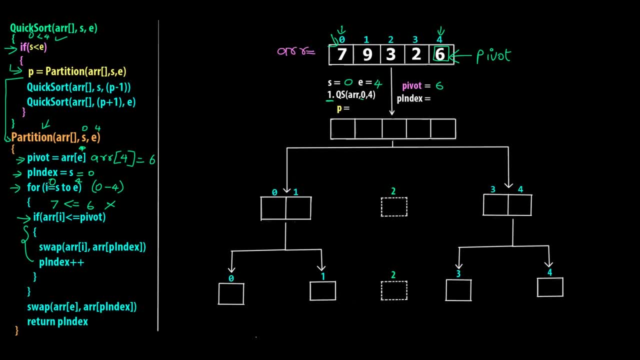 will come outside the if block again. for loop now will become plus, plus, because it is a for loop. It is running from zero to four. So let me just erase all these values. So it's running from zero to four, right, And now I has become one. 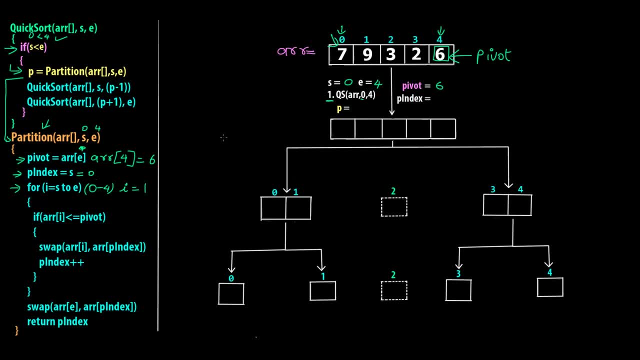 Now we will again go inside for loop. We will say: if ARR of one- which what is ARR of one? ARR of one is nine, Is nine less than equal to the pivot value, which is six. No, So again, this entire if block will not be executed, right? So let me erase this Now. 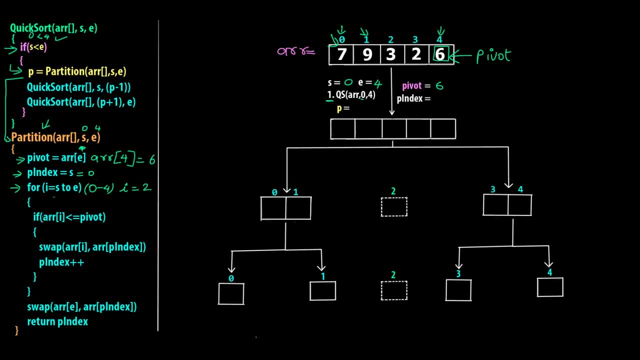 I will become two. We will say: if ARR of two, that is, three, is three less than or equal to the pivot value, which is six, Yes, Now the condition has become two. So this three is less than six. So, according to our strategy, what is our strategy? We want all the elements. 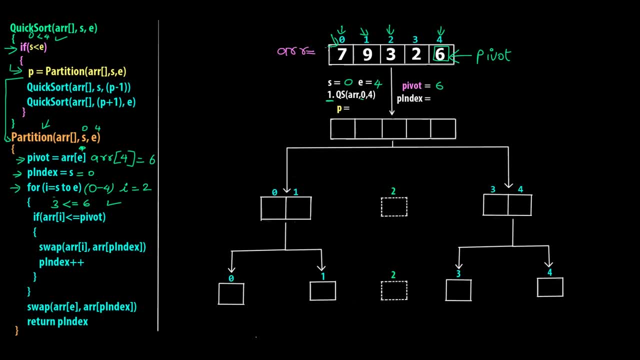 that are smaller than six. that is, smaller than the pivot value to come to the left-hand side of the six value. So what we're doing now is we're going to switch, or we are going to take this three value and put it at the very start of the array because we want smaller. 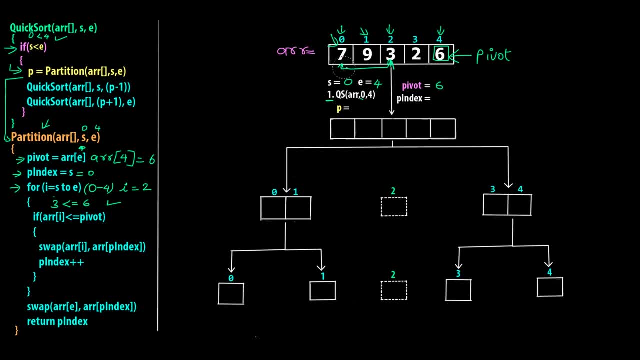 elements to the left-hand side, right. So this is what is happening over here. Okay, So when we go inside the if block, we are seeing swap ARR of I. what is ARR of two? Right now I is two, So ARR of two is three. So swap three and ARR of P index Remember. 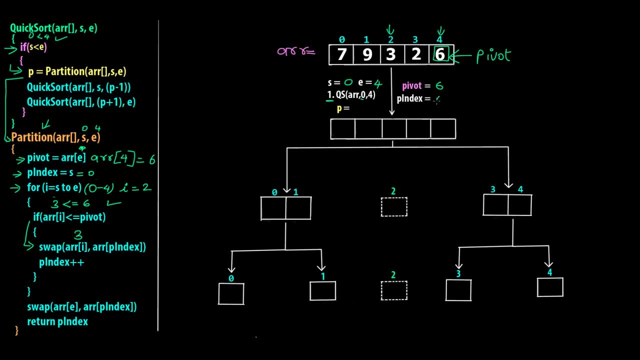 we set P index as zero, right? So let me write it over here also: Initially P index was zero, So ARR of zero is this first position in the array, which is seven. So we have to swap three and seven. So three will come over here and seven will go over here. And the reason: 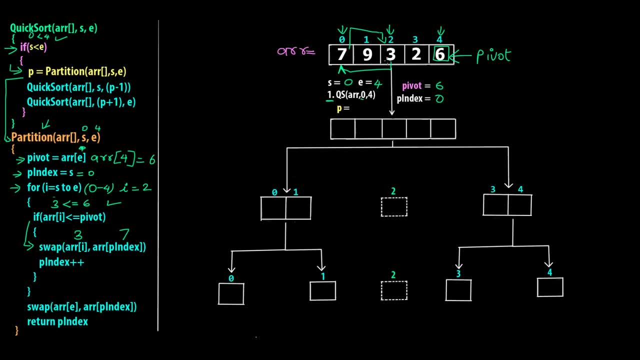 why we're doing is, As I mentioned, three is smaller than six, So obviously three has to come to the left-hand side of the pivot value. So we are already keeping three at the very leftmost value. So after this entire algorithm will execute, three and two will come to the entire left. 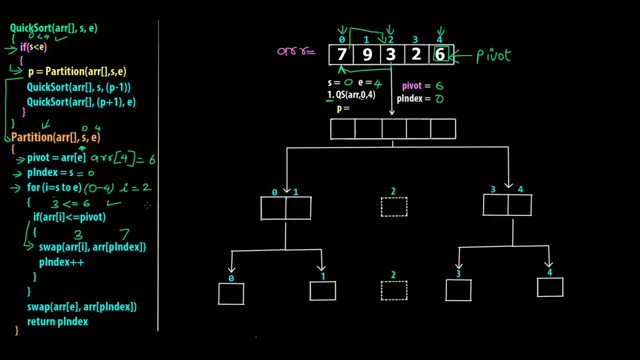 side and seven and nine will shift to the right side. This is the strategy, Okay, So after swapping, let's actually write it over here. Three is shifted over here. Seven is shifted over here. Okay, Let's keep nine and two and six as it is right now, because the 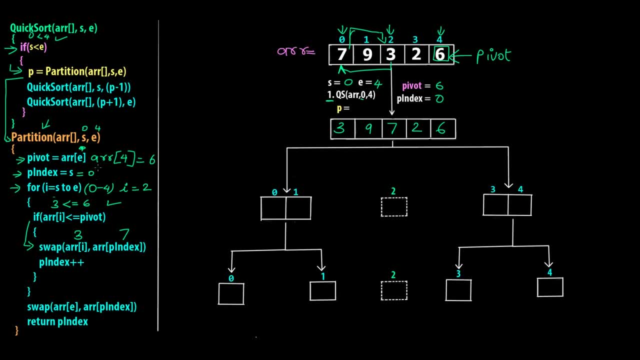 entire algorithm is still not executed. now P index will become plus plus, So P index will now become one right. This is what is happening over here. P index has become plus plus Again. we will come at the end of the if and we will go to the start of the for. 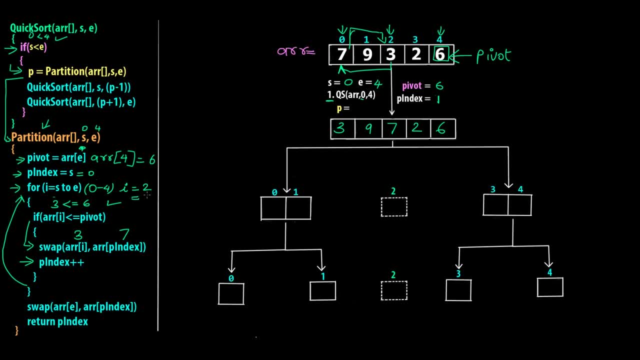 loop. what was I? I was two, So I now will become three. Okay, Let me just erase it off, So I will become three. also, One more thing to note, that is, the for loop will run from: I equals to Yes to E minus one. 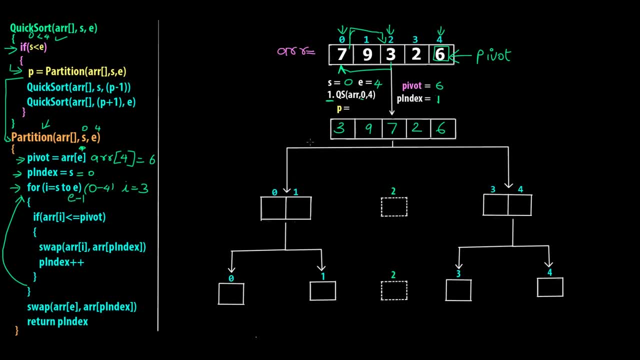 Sorry Is rooted Yeah Rooo. Oh See, if we can, it will still work. It's still learning the to Irish words. now, okay, and not e, because the last element obviously is the pivot. so we only want to compare 7, 9, 3 and. 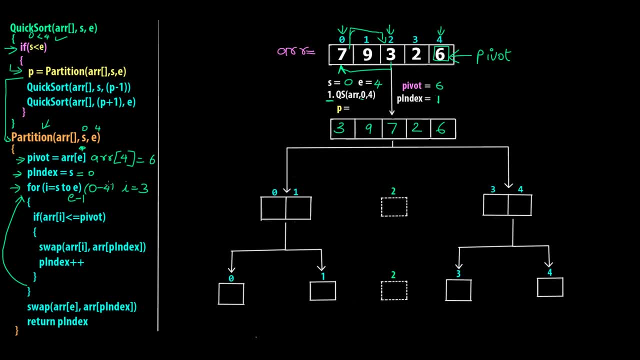 2 and not the last pivot value with itself, right? so this will run from 0 to 3. only so i've made a little mistake over here. it is e minus 1. i hope you guys rectify it, so now i will become 3, okay. 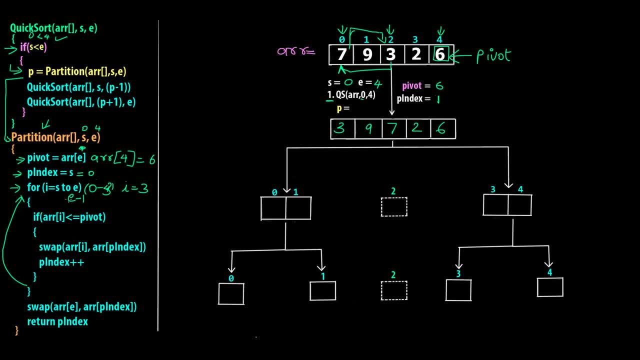 and now we are again going to check if error of i, which is error of 3, what is error of 3 over here? it is 2 and you can now use this new, newly created array because we have just swapped 3 and 7. so now, 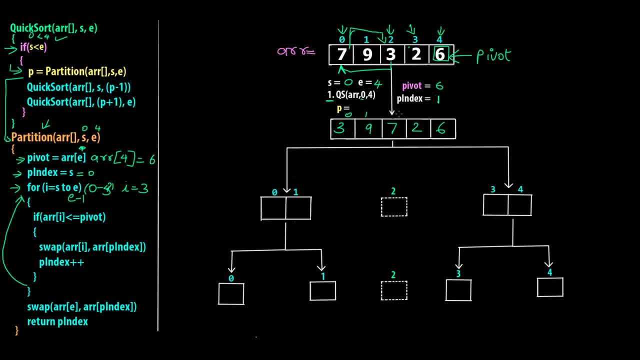 all the comparison should happen over here. so this is 0, 1, 2, 3 and fourth index position. so we are checking error of i, which is 3. so at third index position we have value 2. so is 2 less than equal to the pivot value. what is pivot value 6? yes, so we'll again go inside if now we are saying swap. 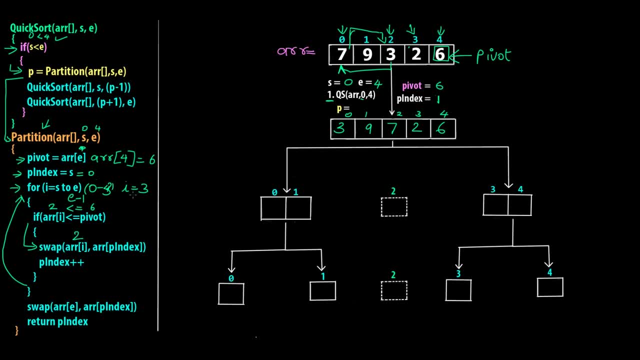 error of i, that is 2, because error of 3 is 2. we have to swap this with error of p index. we just incremented p index by one value and now p index has become 1. what is the value at 1 position? right now it is 9. so now, 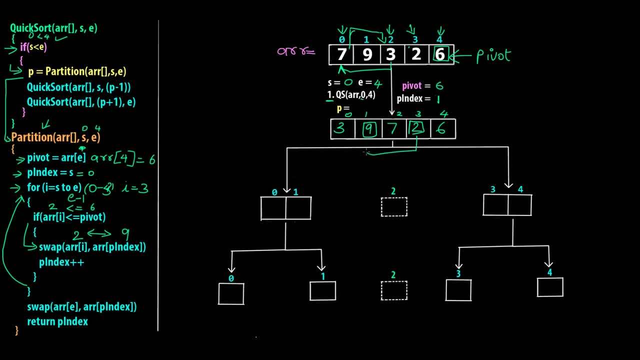 we are swapping 2 and 9, right, so 2 will come over here. 9 will come over here. let's do the swapping. okay, so the swapping is done. 2 has come over here. 9 has come over here again. p index will be incremented, so now p index will become: 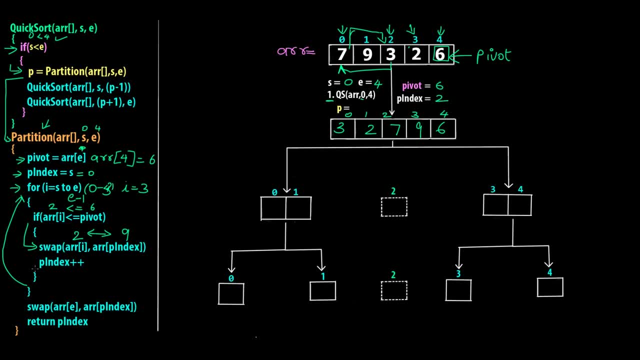 2. right, this is p index plus plus. so we'll come outside. if we will come at the end of the for, for will get incremented and i now will become 4. so obviously the for loop will not execute because this for loop is going to run from 0 to 3 and not 4. the last value obviously is the pivot value. we 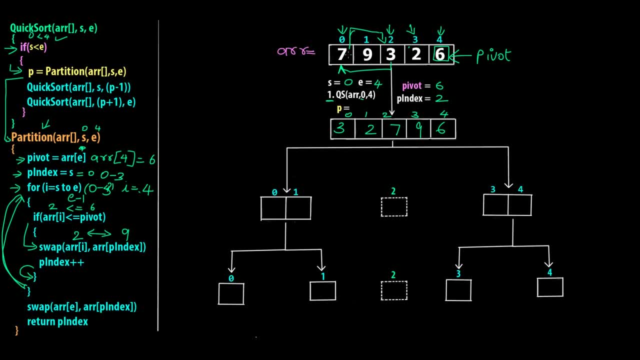 don't have to do the comparison for this pivot value. we have to compare all the remaining elements with the pivot value, right? so that's how the comparison will happen. now we will exit out outside the for loop to the last swapping. so if you've understood this so far, step by step, 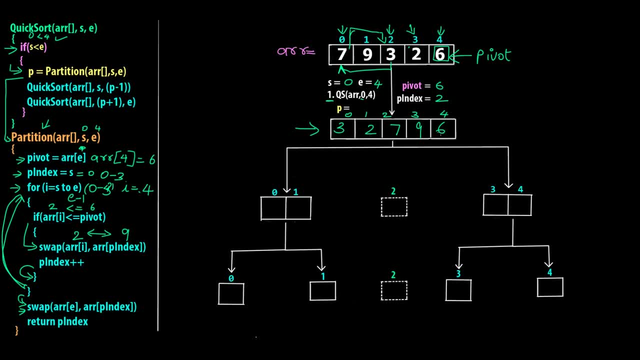 we have arrived at this array: 3, 2, 7, 9, 6. our pivot value 6 is still at the end of the array. so what we did in this partition function so far is all the elements that are smaller than the pivot value 6 we have brought to the left hand side. you can see 3 and 2 are to the extreme left. 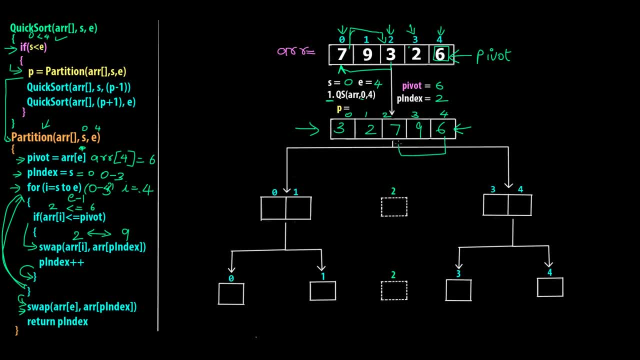 now the only thing remaining is to take this 6 and put it at the position of 7- 7, such that once you do this, 6 will come over here, and then we will satisfy the condition where we were saying that we want all the elements smaller than the pivot value should. 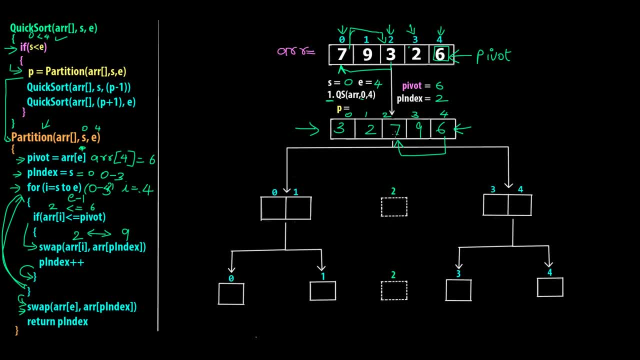 be on the left hand side, because when 6 will come over here, 3 and 2 are smaller than 6 and 7 will go over here, so 9 and 7 are larger than 6. so that is the strategy, right? so this last swap is saying swap arr of e. what is arr of e is the last element, which is 4, which 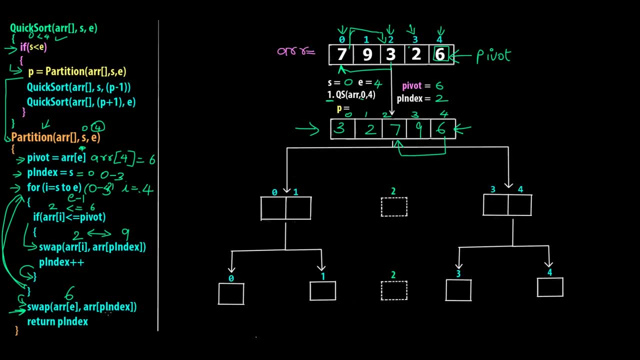 is the pivot value. so swap 6 comma arr of p index. now, remember, p index has come to the point of 2, so we are having index position 2 over here, that is 7. so 6 and 7 is now swapped. so that's. that's the reason why we want p index to keep a track of the positions in. 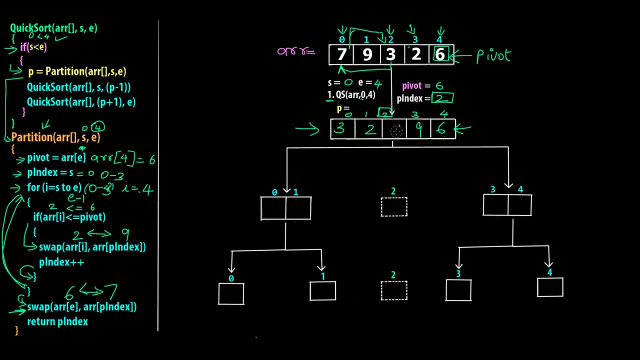 the array. ok, that's the purpose of p index. so now we will swap 6 and 7, so 6 will come over here, 7 will come over here and this is the last swapping that is happening and ultimately we will return p index. what is p index over here? it is 2, so this is returning p index and remember we had called partition. 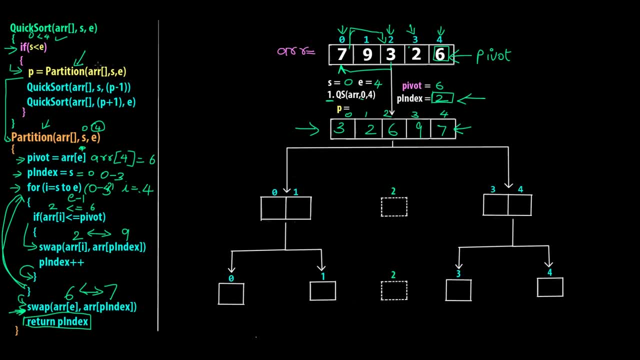 function over here in the quick sort function and partition function is on the right hand side, which means that it is going to return a integer value and it will be stored in this partition p variable. so p variable is waiting for a integer value, which is going to be the 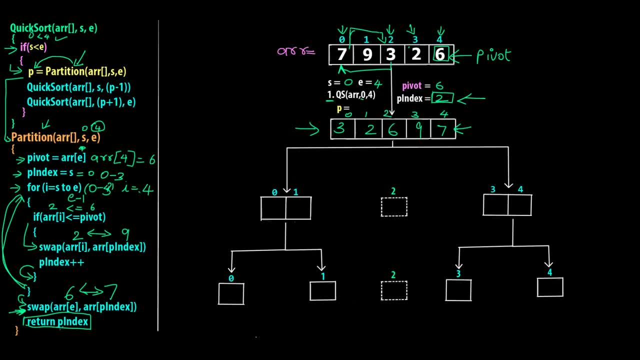 index position where the partition is going to happen, and that is this p index. so p index is 2 and it will be returned from this partition function and it will be stored in this p variable. okay, so this is one entire iteration of partition function and this will result in p value of 2. 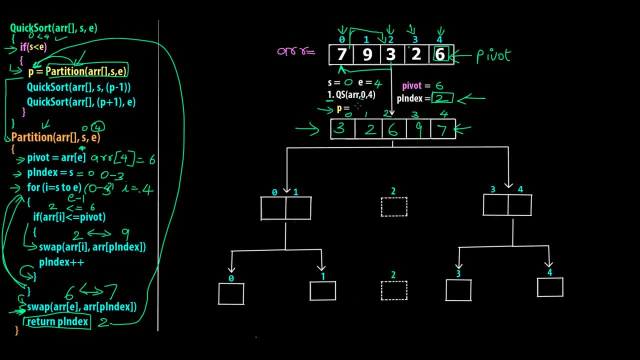 so this p- over here in yellow i have marked this value- will become 2. okay, so after the one full iteration of the partition function, we are getting this array: 3, 2, 6, 9, 7. so the only thing that has happened over here is the value that we selected as pivot has come to the proper position. 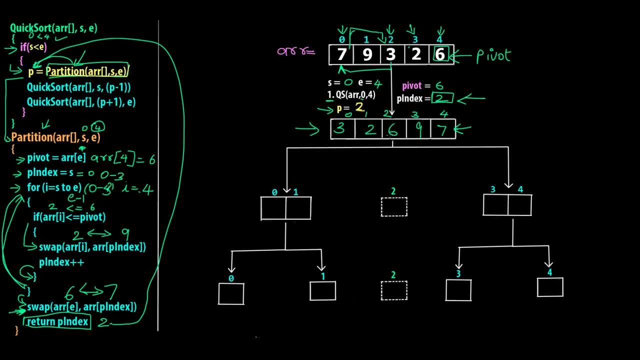 in such a way that all the values to the left hand side are smaller than the pivot, all the values to right hand side are larger than the pivot. now, if you observe, obviously this array is not sorted. 3, 2, 6, 9, 7 is not sorted in ascending order, or descending order, in fact, is not sorted at all. 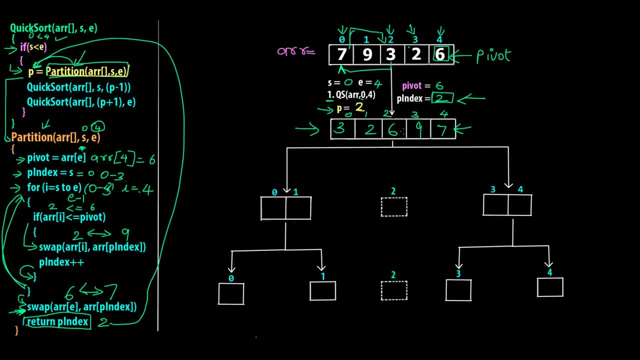 we want to sort it in ascending order, so it should be 2, 3, 6, 7, 9, right, so right. so right now it is not sorted. obviously we are only at step number one. we just gave one quick sort call. so in that first quick sort call we just called the first line, first partition function, and it has returned. 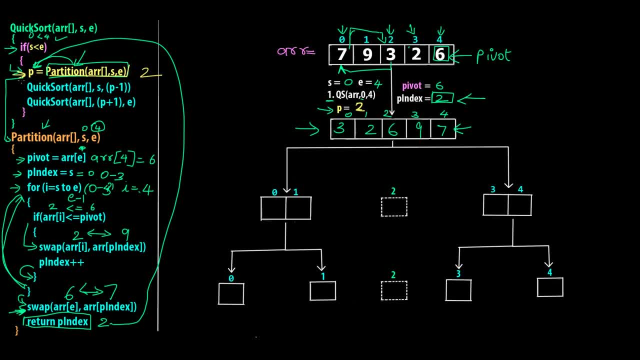 a value of 2. now the first quick sort call will continue to the second step. but second step over here itself is a recursive quick sort call, so let me just first erase out some content from this, otherwise it is going to get very cluttered. okay, so we are at step number two of the first. 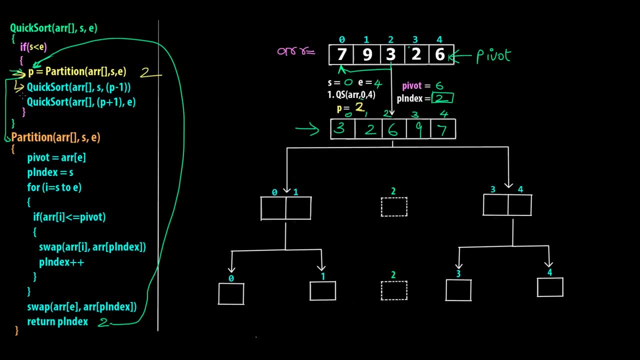 quick sort call and step number two of the first quick sort call is a recursive call to itself, right? so in this case, what will happen is this first quick sort will now be paused. okay, so the first quick sort function is calling another quick sort. obviously, it will go in the pause state, so 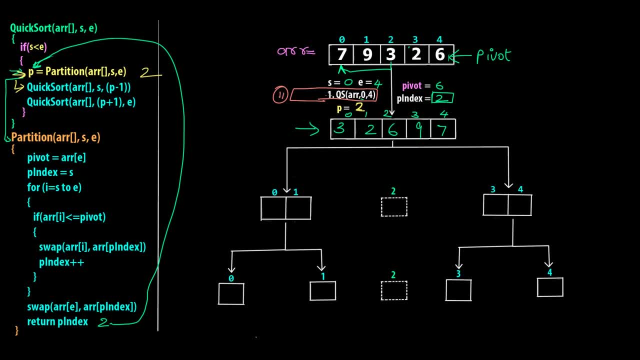 that is how recursion progresses. I hope you know. this first quicksort call is calling second quicksort and it is pausing. in the second quicksort call we are passing the same array. we are passing the start index as s only s is remember it was. 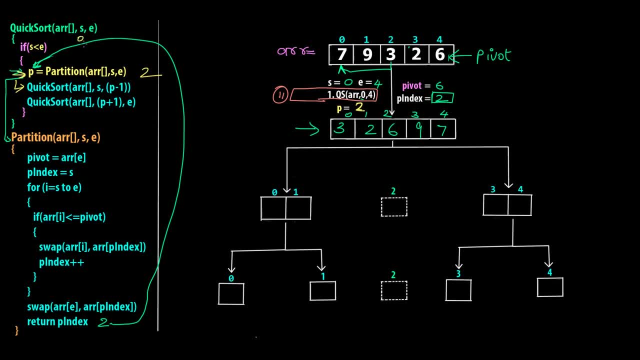 zero. so let me just write it over here: zero and index was four, right, so you can see it over here also: zero and four. but for the end index we are saying p minus one. now we just got the p value as two from this one partition function call. so two minus one is going to be one. so for this quicksort: 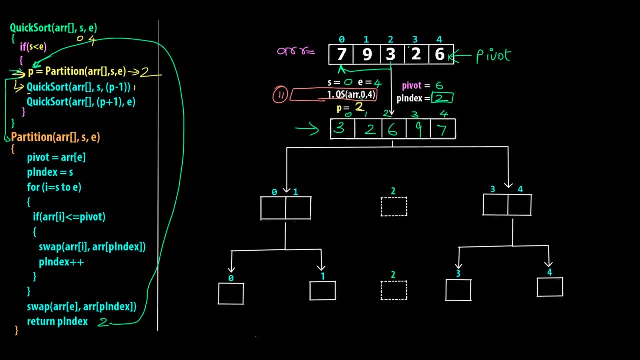 that is the second quicksort call. we are passing the same array, but start index s is going to be zero and end index is going to be p minus one. that is one, okay, so end index is equal to one. so this is how the second quicksort call will look like. so first quicksort call is paused and 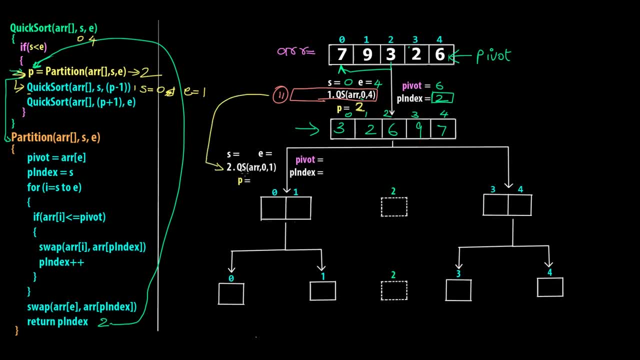 we are giving a call to the second quicksort. qs represents second quicksort. start index, as i mentioned, is zero and index is p minus one, p. we just got us two, so two minus one is one. okay, so we are passing arr zero and one, so a second quicksort is called. now let's start from the scratch. so i'm going to. 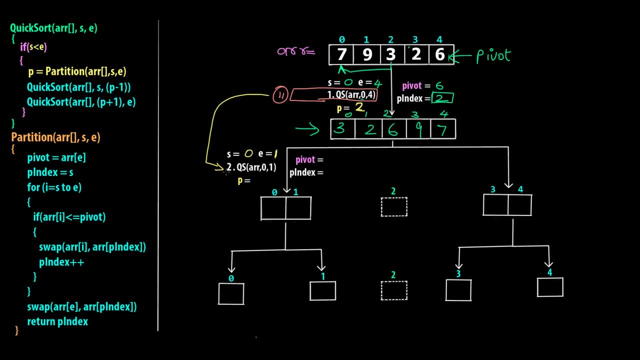 erase this. okay. so first quicksort, as i mentioned, is called second quicksort. we have passed zero one and now this is going to be zero and comma one. so again, starting from the very first step of quicksort function, it's a recursive call. we are saying: 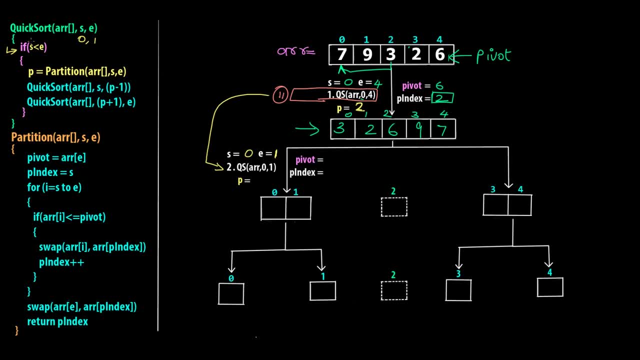 if s is less than e, s is zero, e is one. obviously zero is less than one. so it is true. so we will go inside the if block and again we are calculating a new partition value by saying p is equal to partition of arr, s and e. now, this time s is zero but e value is one. okay, so partition is giving a. 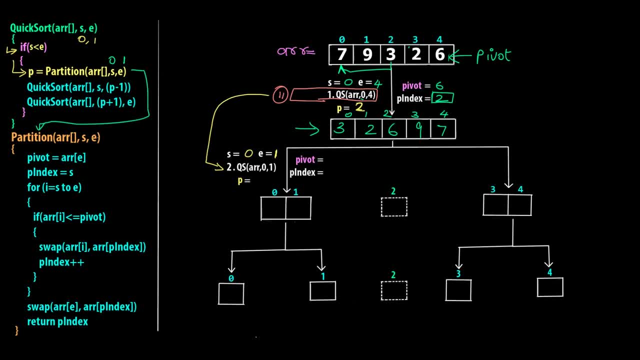 call to this function. in this we are passing s as zero, e as one. so that's the way it is going to be. only difference, so zero and one. now we have to calculate pivot, p index and p inside this partition function. so again the same thing- repeat story- is happening. so pivot over here is arr of e. 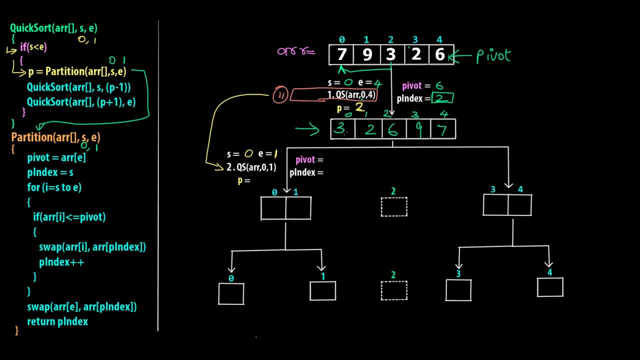 this time, e value is one, okay, and now we have to use this array as the fresh array. we cannot use the previous array. we've already made changes to the same array. remember: this is an in-place sorting algorithm, so every step is happening on the same array and not any temporary array. 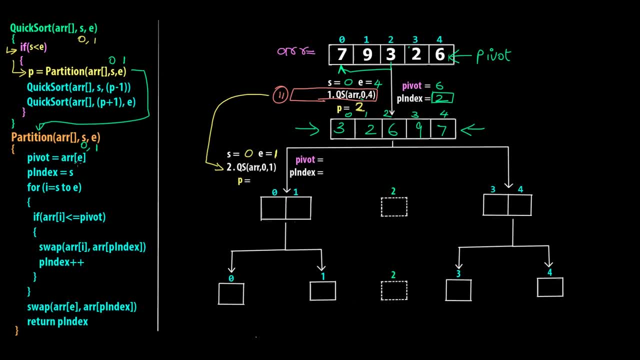 so now we have the fresh array of three, two, six, nine, seven. what is arr of e? it is arr of one because e this time is one. you can see i've written e as one arr of one, for the fresh array is zero, one, two, three, four, one is two, right, so this is going to be two. so pivot this time is two. so essentially, 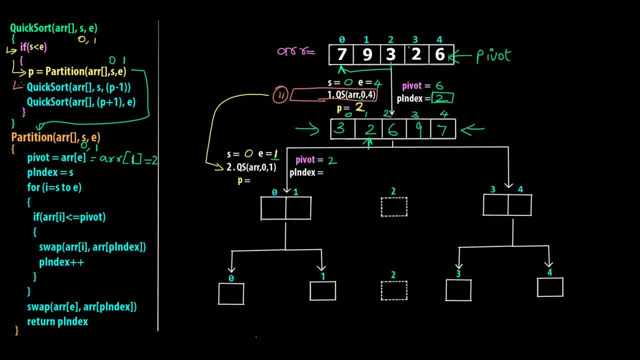 what we're doing is we are applying quicksort, because we are at this step of the first quicksort. we are applying quicksort on the left partition, so we got six in the middle after the first step. so the two parts that we have is: this is one part and this is second part. so we are applying. 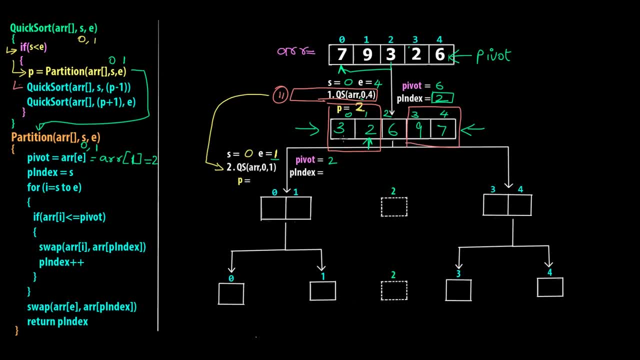 another quicksort call which is going to happen to the left hand side. so for the left hand side, that is left sub array or left sub partition, which is the last element, obviously two. hence we are selecting the arr of e, that is arr of n, index, that is value two, which is stored inside the pivot. 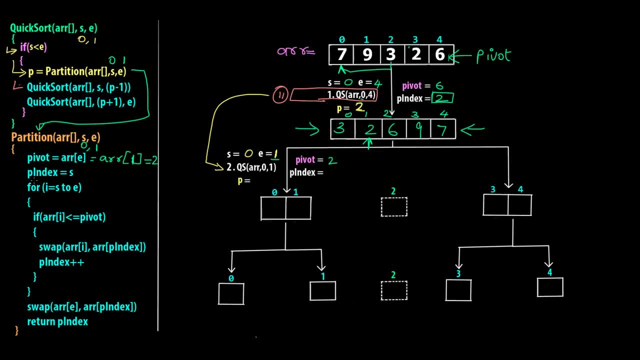 so pivot is done. pivot value is two. next is p: index is equal to s. s is obviously zero. so p index initially is going to be zero. now we are again going to say: for i is equal to s, to e minus one. so this is e minus one. let me actually make this change over here itself right now. okay, so i is. 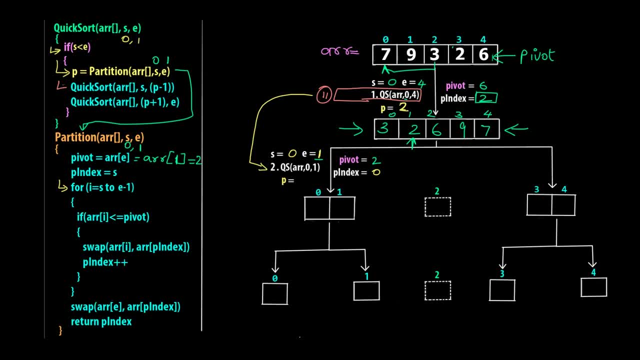 equal to s, to e minus one right. so what is s? s is zero, e minus one. e is one, e is one one, s one is zero. so from zero to zero. it means that this for loop will run only one time, because we only have two elements in the left sub array, that is, left partition. 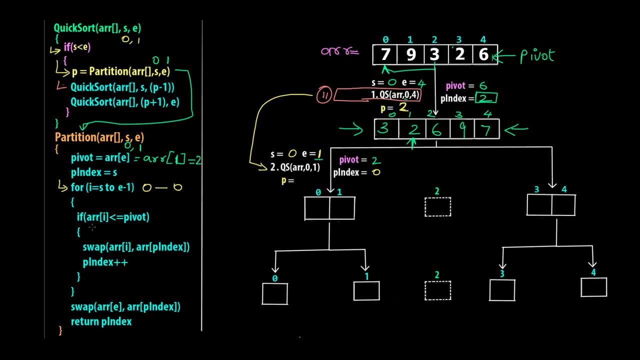 in this case. so in this case we are saying: if arr of i, what is i? i is zero initially, so arr of zero is three, right, arr of zero over here is three. so is three less than or equal to the pivot value. what is the pivot value over here for the second iteration or second quicksort call? it is two. 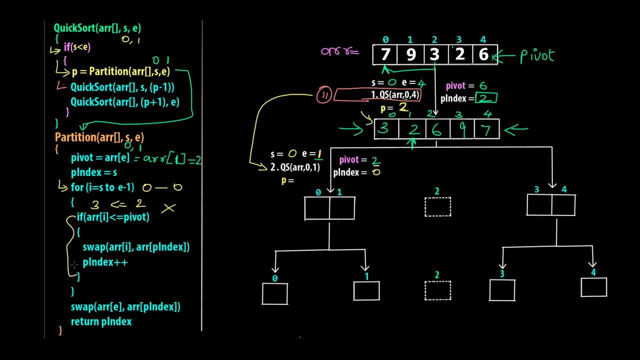 is three less than or equal to two. no, so this entire if block will not be executed. we will come at the end of the. if we will go at the for four will become plus plus i will become one, and we are only running from zero to zero. so this for loop also will stop running. so now we will. 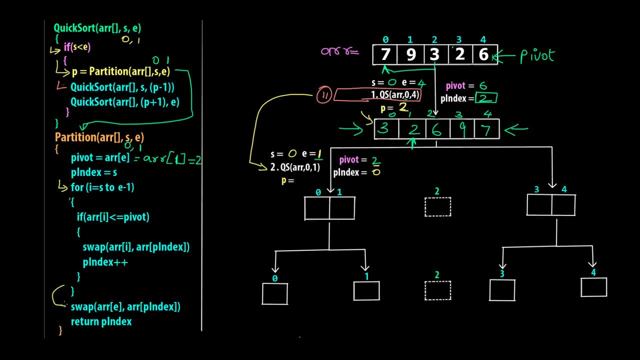 come outside the for loop. so coming outside the for loop is the last step of the last swapping, and the last swapping says arr of e. what is e one? what is at index position? one, two. so swap two with arr of p index. what is p index? p index we set as p index is equal to s, which was zero only. 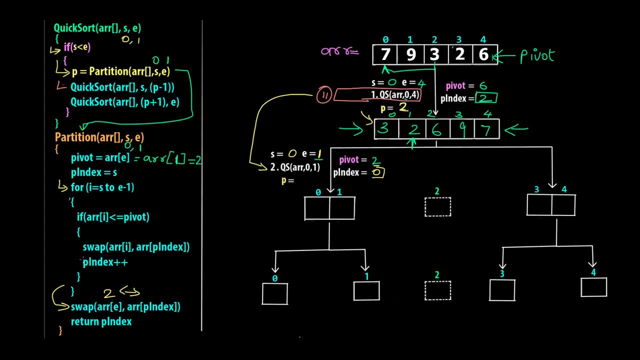 so p index never got incremented because we did not go inside the if block. so what is the value at zeroth index? it is three. so you have to swap two with three. so two will come over here, three will come over here. so that is what is going to happen over here, so i'm going to write it: two. 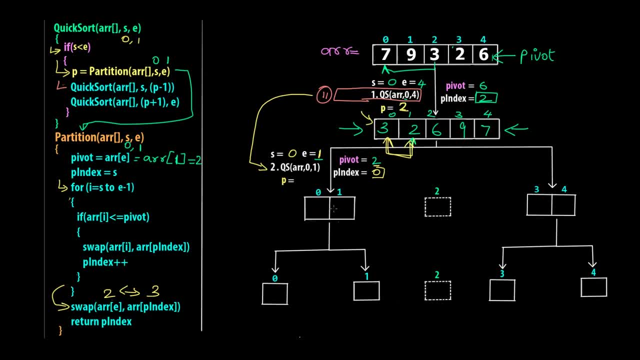 and three. let me write it in green. so two is over here, three is over here. let's keep this six as it is. by the way, these are not separate sub arrays, okay, so i've just marked them zero, one, two, three and four. so this is the same arr only, but i have represented it. 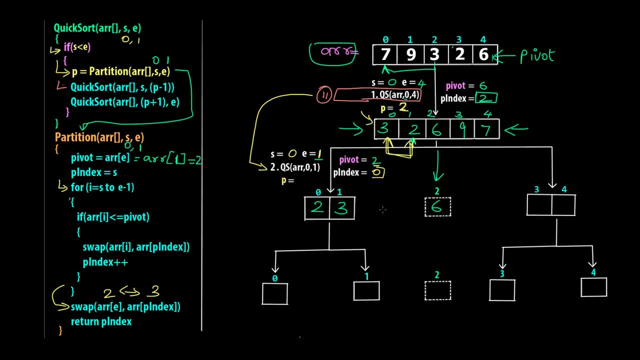 in separate blocks. ultimately it is the same array, only it is not divided. you can make it out with the index positions also. so six is always going to be in the middle. we've just sorted the left hand side. you can see two and three. so two, three, six is pretty much sorted now. okay. 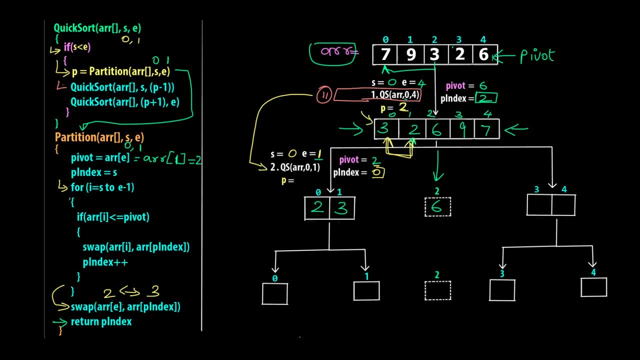 so we did the swap. we will say return index, that is, return p index. what is p index? p index is still zero, so zero will be returned over here and now. it will be stored in the p value of this quicksort call. this quicksort is the second quicksort call, right in the second quicksort call. we are at step. 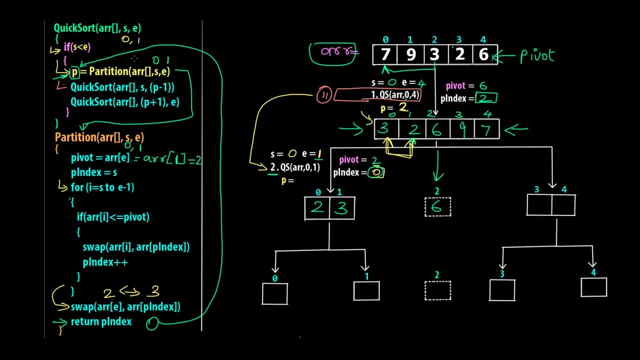 number one, which is get the partition index. what is the partition index? that we got zero, so i'll write zero over here. now we will move to the next step, the second quicksort call. but if you observe, the next step itself is a third quicksort call. 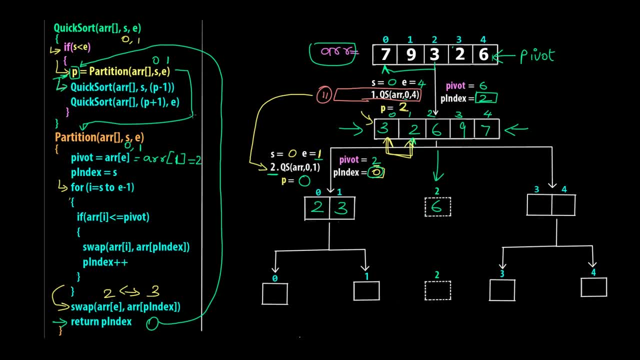 that is a recursive call which is going to apply quicksort to the left side of this subarray. what is the left side of this subarray? it is going to be a single cell element, right? so here the quicksort will be the same array, that is, this entire array, but here the s is going to be zero. 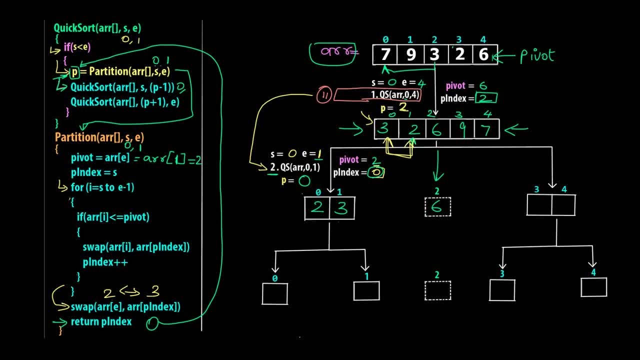 obviously. but now we are going to say p minus one. what is the p that we just got from here? we got p, remember? we just got zero. so zero got transferred and stored in this. that is what i showed over here with this entire arrow. so zero minus one is going to be minus one. so a third quicksort call is given. 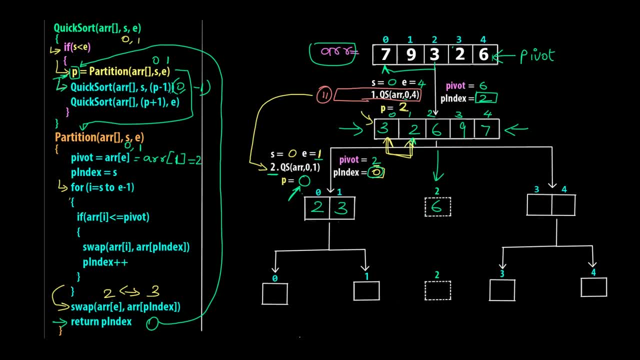 with values of arr, ss zero and e- e value, that is, n index- as minus one. now obviously we don't have minus one as index values, so let's see what happens. so of course, third quicksort call is called, which means the second quicksort is going to go in the pause state. 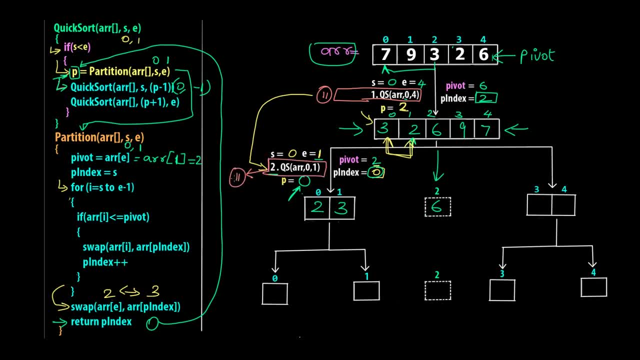 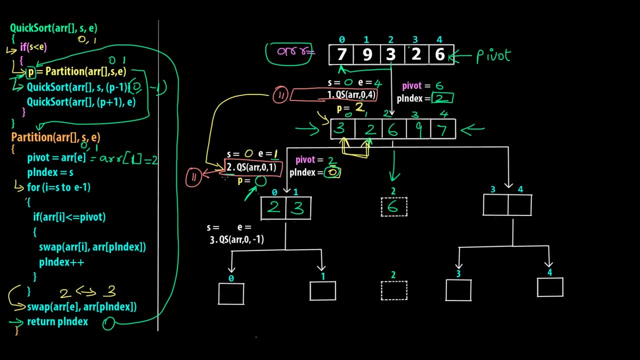 this quicksort will now become paused and the third quicksort call is given. so let's see that call. so second will be paused and a third quicksort call is given, and this is how it looks like: start index is going to be zero and index, as i mentioned, is p minus one p. we just got as 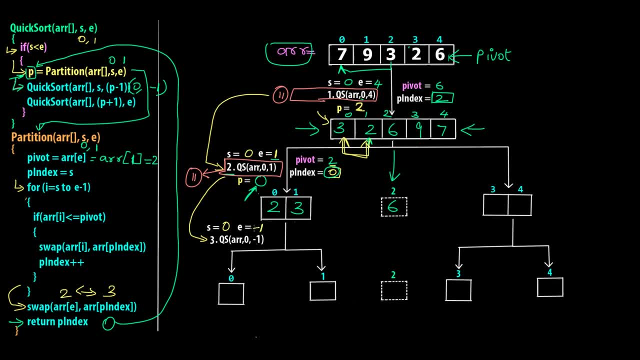 zero. so zero minus one is minus one, so n index is minus one. so again, this entire quicksort will be called. so let's start from the scratch. so for the third call, that is, third quicksort call, the array is passed as it is, but we are passing. 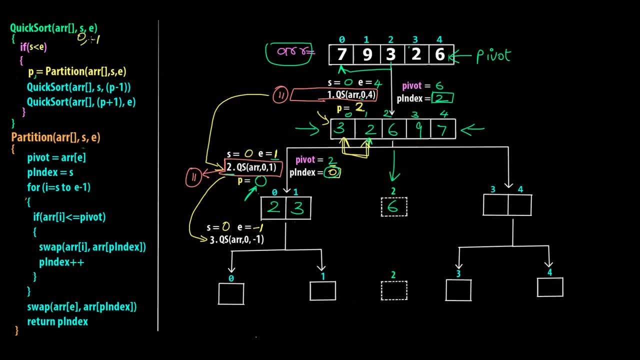 start index as zero and index is minus one. obviously minus one does not exist in array indexes and that is handled in this if condition, this if condition says: is s less than e? what is s zero? what is e minus one is zero. less than minus one? no, and this is where the recursion breaks. 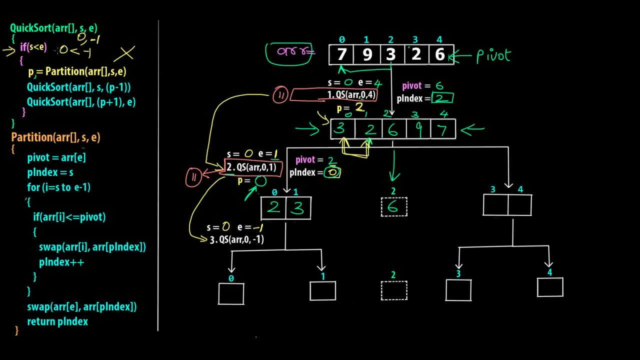 out. so if block has become false, s cannot be greater than the end index. the start index can never be greater than the end index. s is zero and e is minus one, which means start index has become greater than the end index, and this condition will never exist. it is an invalid condition. 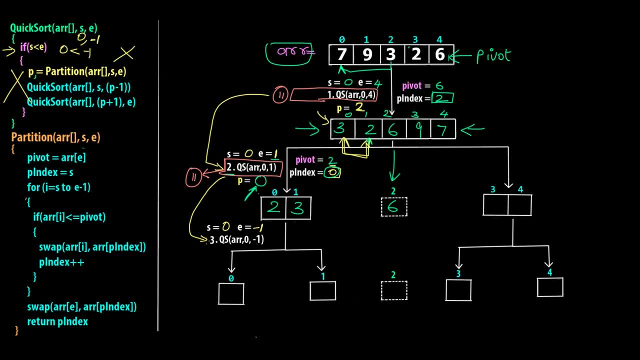 so now the entire if block will not be executed and quicksort will stop. that is this entire if block will not be executed. we will come at the end of the function over here, which means this quicksort has done its execution. this is a third quicksort. 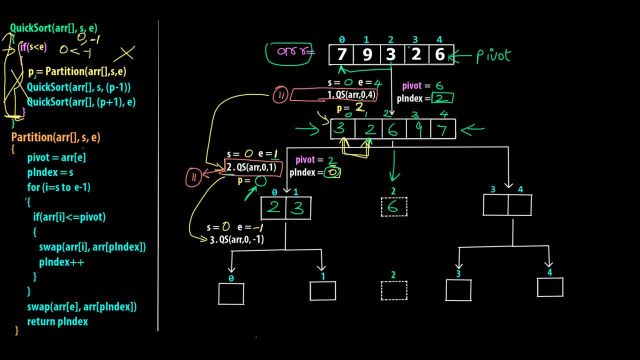 call. so who called the third quicksort the second quicksort? right, so now we will go back, which means from third quicksort we will go back to the paused second quicksort. so now this will no longer be paused, it will start its execution again. remember, the second quicksort has paused at. 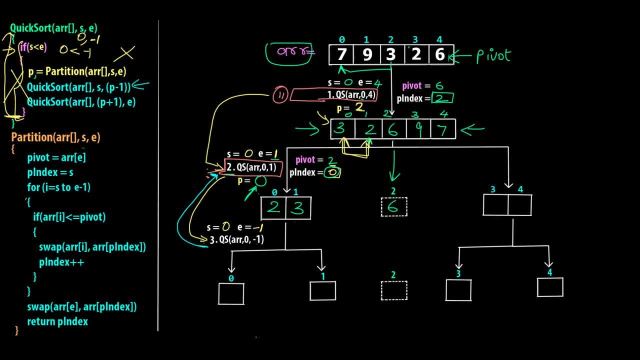 step number two. that is the third quicksort call. so it will go to step number three. and step number three is one more quicksort call, but this is for the right side of the partition, or the right most partition. So over here at this step we have ss0 and es1.. So we will give one more quicksort call. that is this. 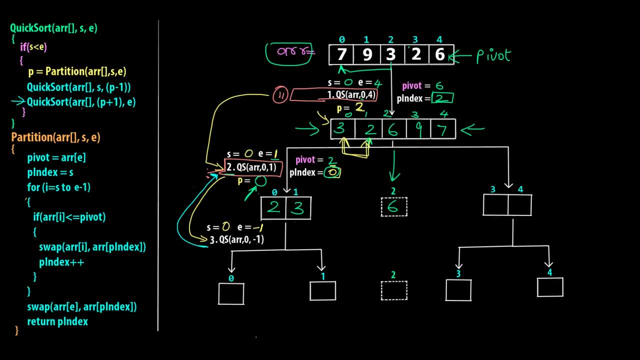 quicksort call and this quicksort is gonna say the same array, but the start index is p plus 1.. So at step number 2, or at this level of quicksort, what is p value? p value is 0.. So 0 plus 1 is 1.. What is e value? e value is 1.. We will pass as it is. So a fourth quicksort. 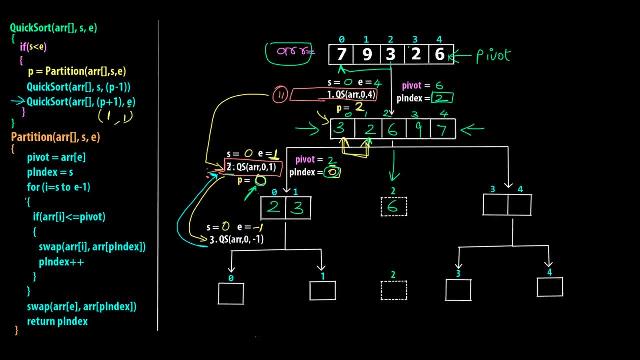 call is called from second quicksort call. So again this will become paused. Let's see what the fourth call is. In the fourth call, as I mentioned, the start index is 1, that is p plus 1.. p is 0 over here, So 0 plus 1 becomes 1.. e is also 1.. So we are saying quicksort. 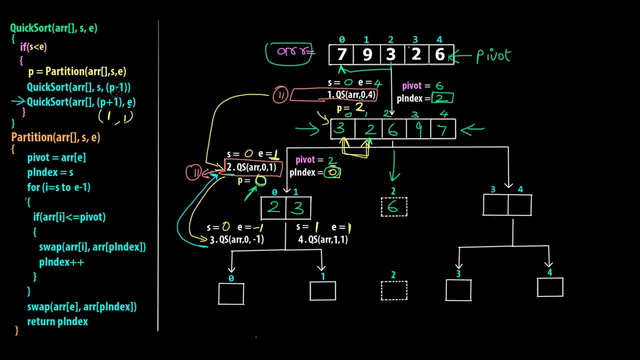 of arr. So a new quicksort is called. Let's see what this quicksort will be. So s is 1, e is 1, in the condition. if s less than e Is 1, less than 1? No, 1 is not less than 1, right. So again, this entire. 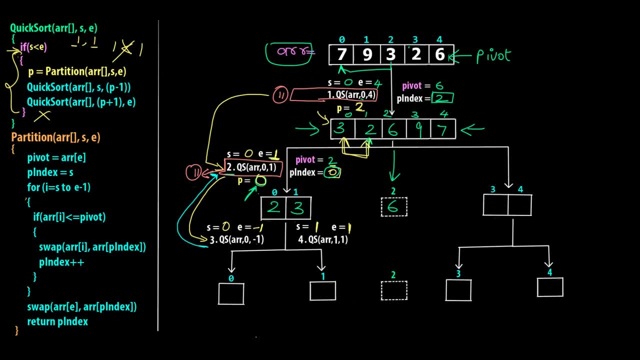 if block will not be executed, which means quicksort will not go into a recursive call, One more recursion will not happen. So this quicksort will be done. So this second quicksort had called fourth quicksort And fourth quicksort is done, its execution. So it will come back now to this. Okay, And 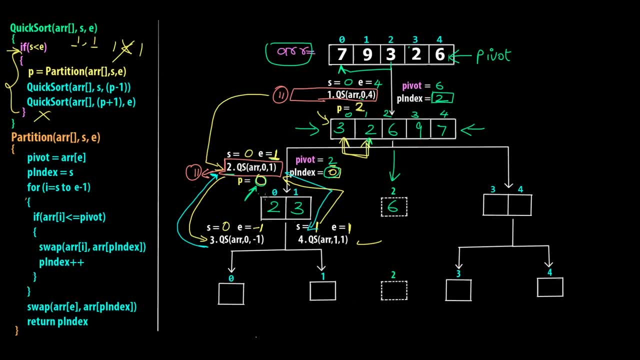 2 and 3 will remain as it is. So nothing happened to 2 and 3.. They were as it is because the recursion broke off at third and fourth quicksort call. They did not go inside, We did not call the partition, We did not call multiple quicksorts. So 2 and 3 is already resolved over here also. 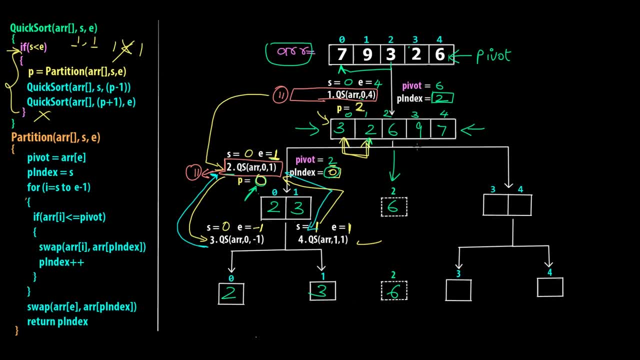 Let me write 6 also. as it is, You can see, on the left hand side, the left branch is pretty much solved. So we will go from first quicksort back to second quicksort. The second quicksort had come to this step and after this step the if block will complete itself. We will come. 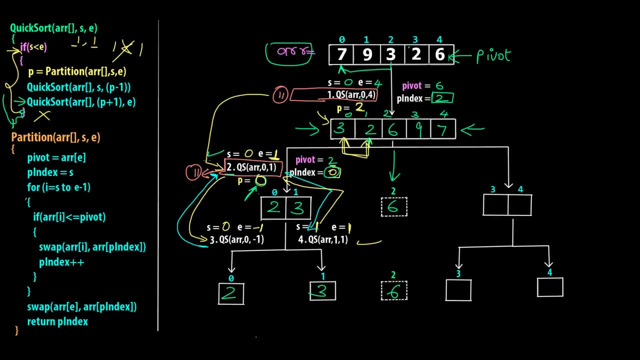 outside this quicksort also. So second quicksort will also be done. So erasing this off Who had called second quicksort First quicksort. right, First quicksort was paused and it called second quicksort. So we will go back from second quicksort to the first quicksort Now. 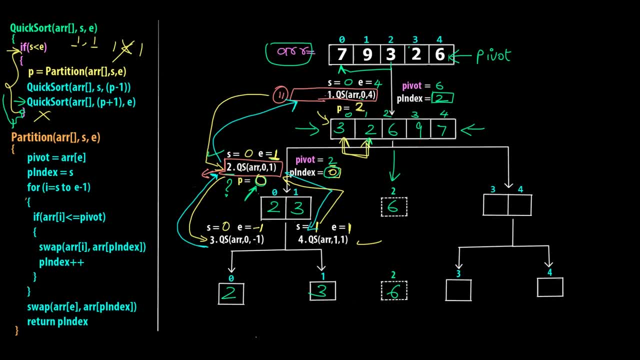 at this level. If we come back to the first quicksort, the first quicksort was paused at step number two, itself right, So it had paused over here. That is, first quicksort gave a call to second quicksort, So first quicksort gave a call to second quicksort and this quicksort is 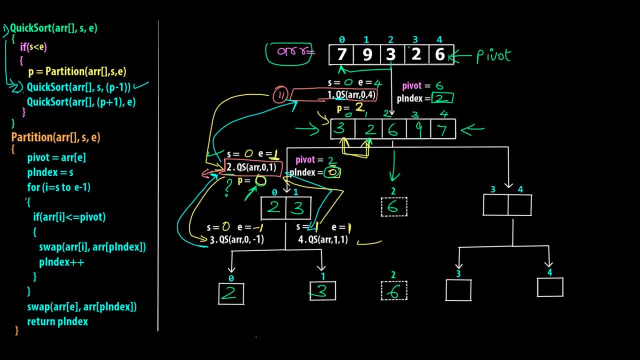 done. now The left hand side quicksort is done, executing. So second quicksort came back to the first quicksort. That is how recursion works. But now it will move to the next recursive call. But this time the quick sort will be called on the right hand side, So it will be called. 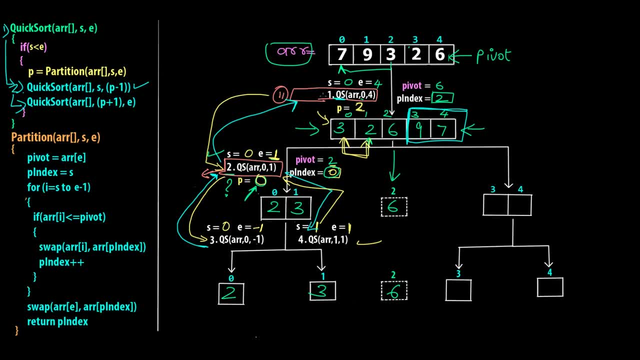 on this sub partition. So at this level, at the top level of first quicksort, we have SS zero and ES four. We also have got the P value of two. So a fifth quicksort call will be given because we've called one that over here, we've called two that is over here, we've 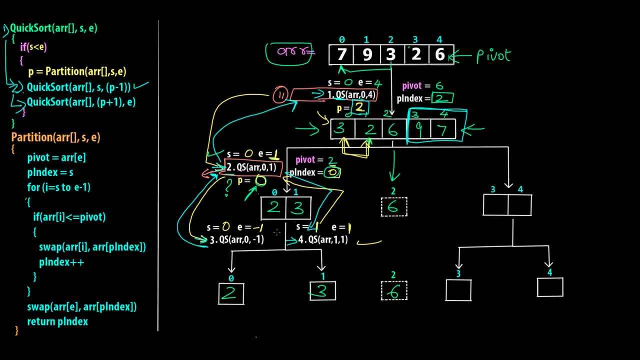 called three and four. So four quicksort calls have already happened. Now a fifth quicksort call will be given, but this time it would be for the right hand side. So we are passing the array. We are seeing P plus one. So at the level one, at the top level, P is two, two. 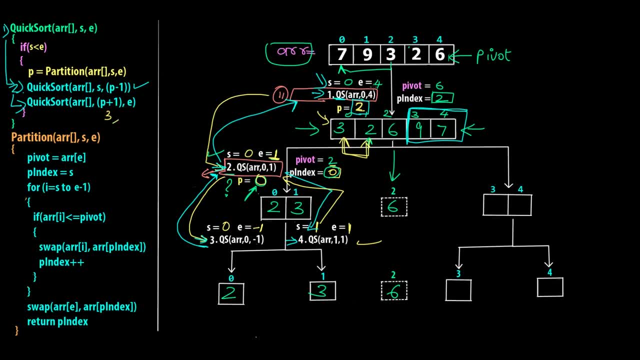 plus one is three. And what is E? E is four at the top level right, So three and four. So three and four are these two indexes. So we are only going to call quick sort for these two values. So let's see how the fifth call looks like. Okay, So now the first quick sort. 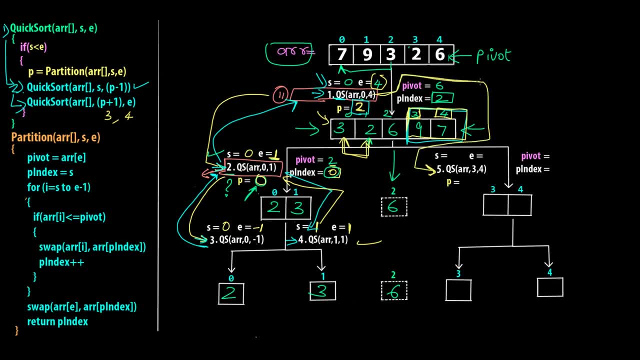 is giving a call to a fifth quick sort recursively. So I hope you are getting how the entire algorithm is progressing, how the recursion is working. in the fifth quick sort, The start index is three, The end index is four. So now let's actually calculate, or let's start from the 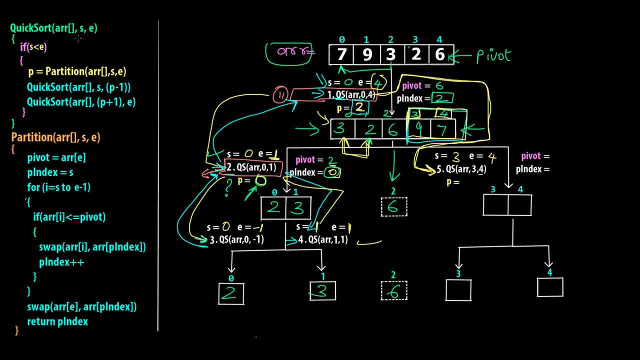 scratch or start of this quick sort function. So start: index is three and index is four. is three less than four, Yes, So we'll go inside the if block. Now, again, the partition function will be called At this level. we have to calculate pivot P, index and everything. So let's start with. 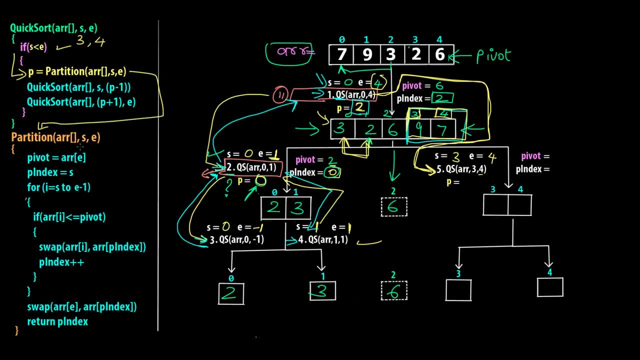 the partition. So partition function will be called. We'll come over here. S is three, E is four. Pivot is error of E. E is four. What is error of four? over here? It is seven. So now pivot value becomes seven. P index is equal to S. S is three. right, S is three. 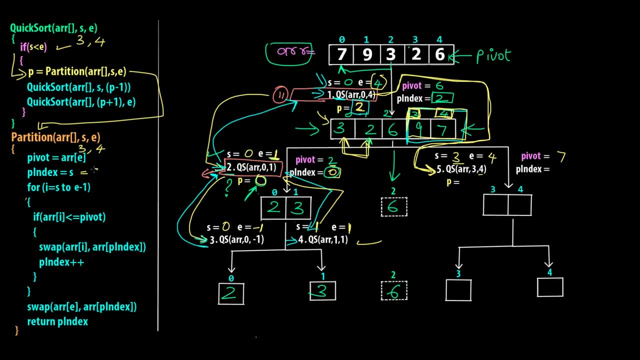 So value at three is nine, So P index becomes nine. Let me write it over here also: P index becomes nine. We are saying: for I is equal to S to E minus one. What is S? S is three. From three to E is four. Four minus one is three. So 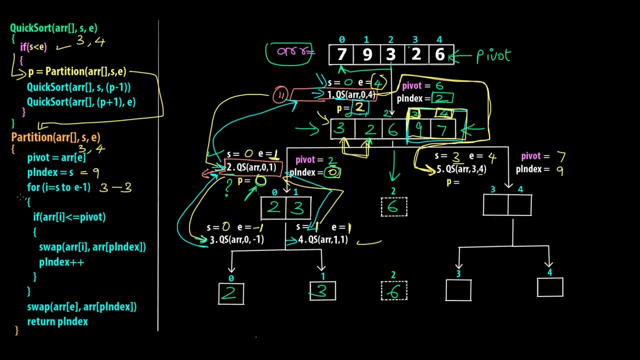 from three to three, which means it will run only one time. This for loop will run only one time. We will go inside. We are going to see if error of I what is error of I. initially I is equal to S, S is three. Error of three is nine, right, So this is error of three. 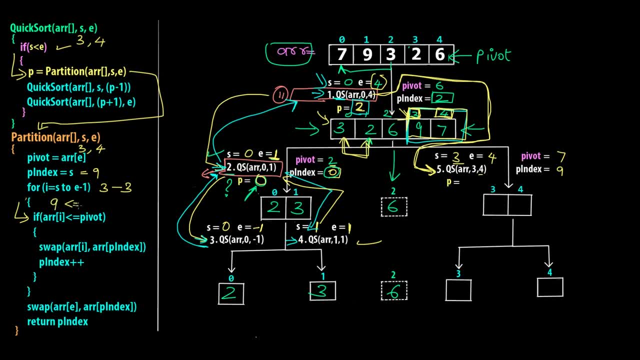 It is going to be nine. Is nine less than equal to the pivot value? What is pivot value? We just said pivot value is seven. Is nine less than equal to seven? No, So this entire if block will not be executed. We will come outside if block. We will go to the start. 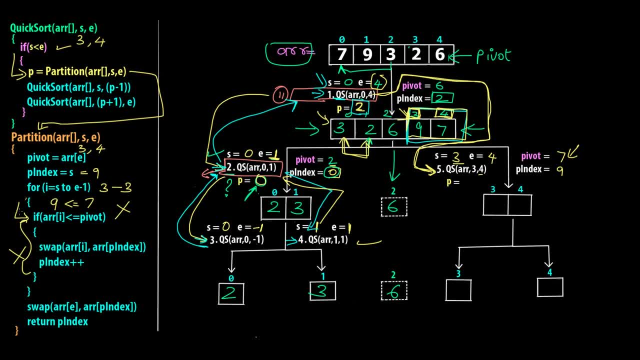 of the for For loop, as I mentioned, is only going to run one time, So we will come outside the for loop to the last swapping And at this swapping we are saying: error of E. What is E? E is four. What is value at fourth position. 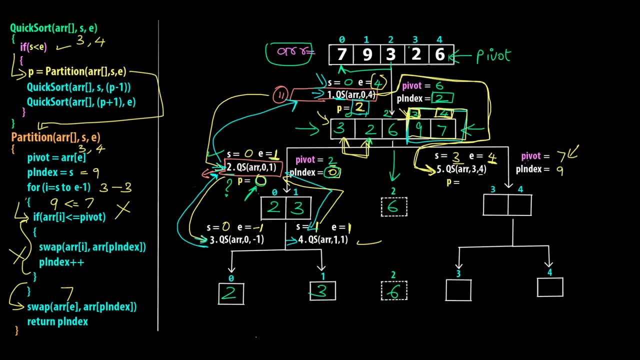 Seven. We have to swap seven with error of P index. P index, as I mentioned, is okay. P index is supposed to be S, Okay, S is basically three. So this is the P index and not nine. So the value at position three- that is error of P index, which is error of three- is nine. 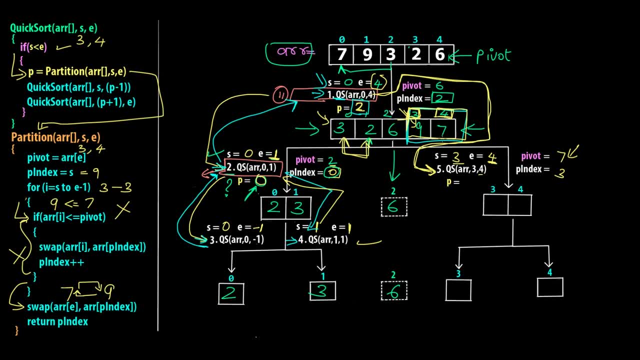 So we have to swap seven and nine, because seven is obviously smaller. So seven will come over here and nine will come over here. So ultimately we will have seven and nine. Let me write it in green because it's sorted. And lastly we will say: return P index. What was P index? P index was three, So three will. 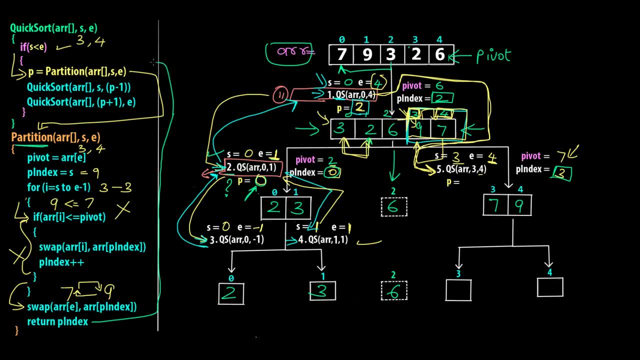 be returned back from this partition function and it will be stored in this P variable. Now we are at quick sort, which is a fifth recursive call. We've just calculated P as three right P index was three. It is returned and stored in the 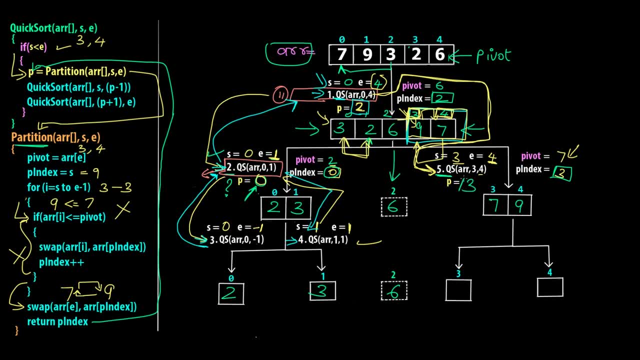 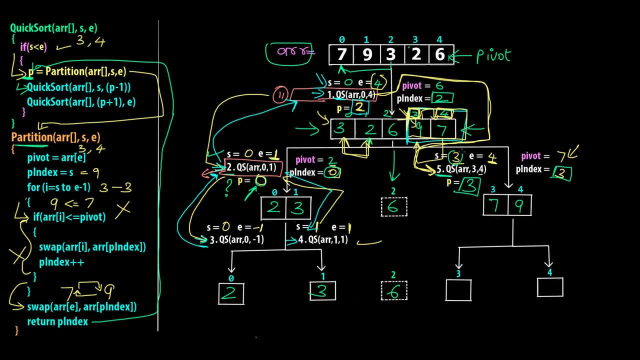 of S and P minus one. S at this level is three, So we'll say three comma P minus p. we just got us three. So three minus one is two. Now if you observe, obviously this quick sort will not execute, because starting index is three and then index is two. Obviously this can. 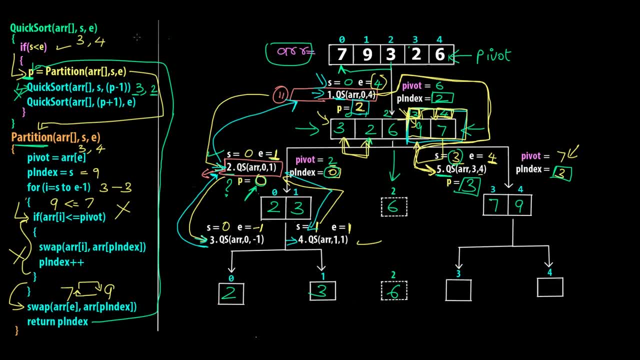 never happen, Right right, start index can never be greater than the end index. so a sixth quicksort call will obviously be given. let's see how that goes. so a sixth quicksort call will be given. so this fifth quicksort will become paused and a sixth quicksort will be called. but here s will be 3 and e will be. 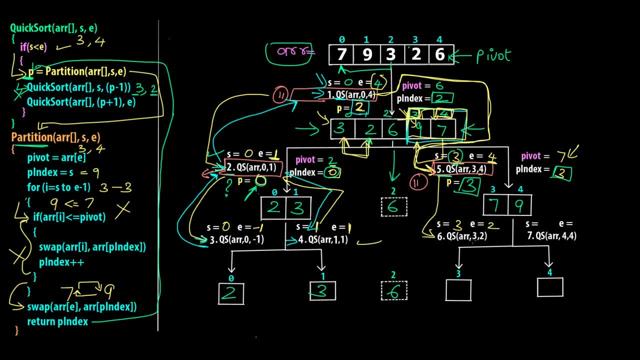 p minus 1, that is 3 minus 1, which is 2. so that's why 3 and 2. but in the if block, when we call the quicksort again, we will compare: if s is less than e and over here s is 3 is 3 less than e, which is: 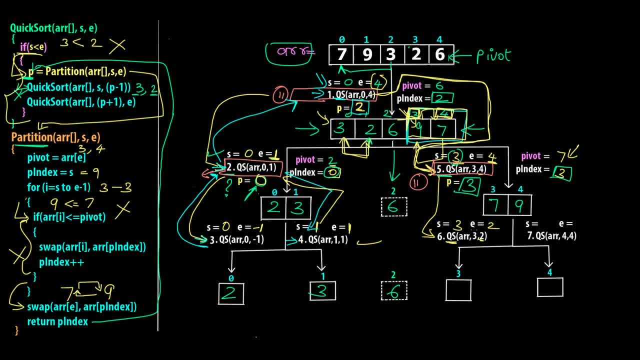 2. no, so this entire quicksort will not be executed at sixth quicksort call. so this will be done. so this is done and it will come back to level 5, that is, fifth quicksort call. when it will come back at fifth quicksort call, a seventh quicksort will be called from fifth quicksort, which is for: 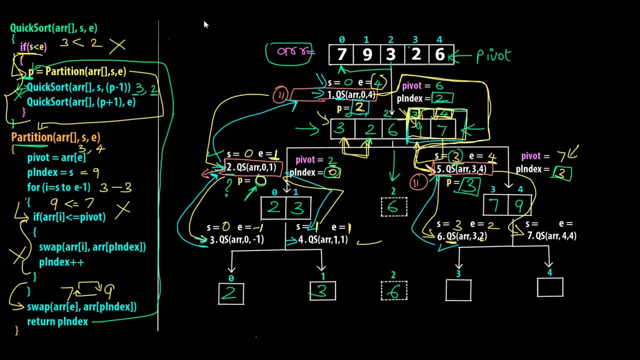 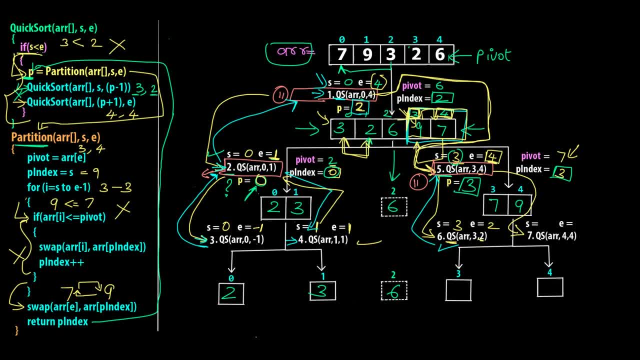 passed. and again in the quicksort we will check if s is less than e, so is 4 less than 4? no, so 4 and 4 will be passed and obviously this quicksort will also be done. so 5 and 9 will remain as it is. they are already sorted. basically, so these last two quicksorts. 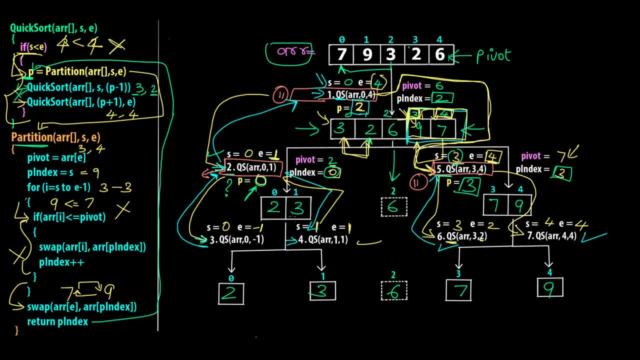 and these two quicksorts were just called for the sake of calling, but the condition was never true, so multiple recursions did not happen. if you give a wrong condition over here, you will go in infinite loop, infinite recursive calls. but anyways, coming back, seventh quicksort will go back to fifth. 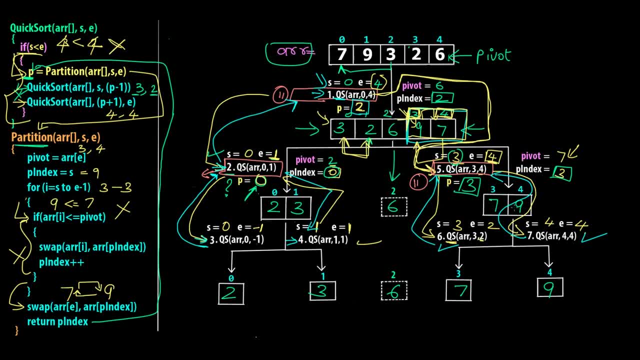 quicksort because fifth quicksort had called seventh. remember that this fifth quicksort was called by the first quicksort and it is still paused. so fifth quicksort will get done at the last step and this will also be done and it will return back to the calling function, which is the very 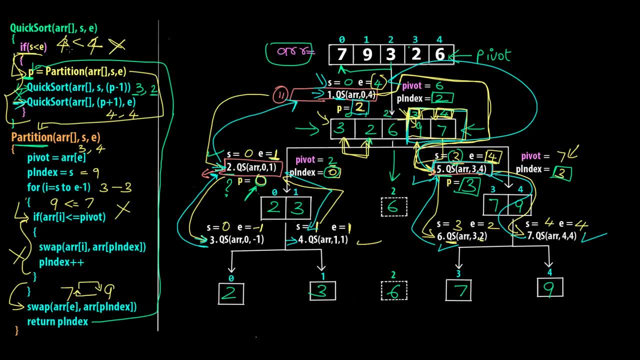 first quicksort. when it comes back to the first quicksort, the first quicksort will also be done, because the first quicksort is done, calling quicksort for the left hand side and the right hand side. you can see it is called quicksort for the both sides and it has become very cluttered. 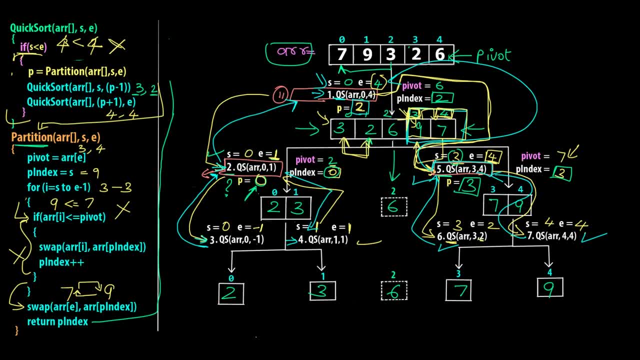 right now. i know it is looking very shabby, but ultimately, if you see at the end, the result is what we've got is a sorted array. if you observe these values, two, three, six, seven, nine are in a sorted way and this is the same array that. 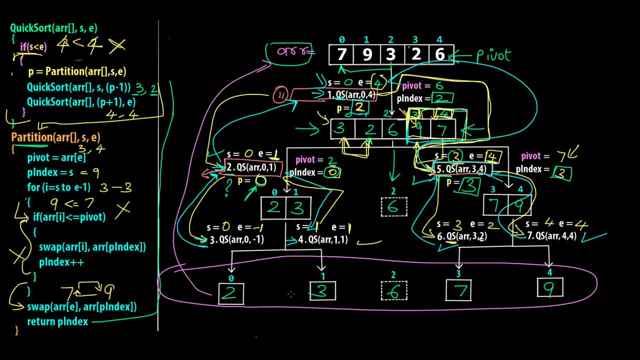 we had arr, only i have just separated or added space in between, but ultimately this is going to be two, three, six, seven and nine. okay, so this is how the entire quick sort sorting algorithm works. these are the two different functions and this is how recursion works and the partition function. 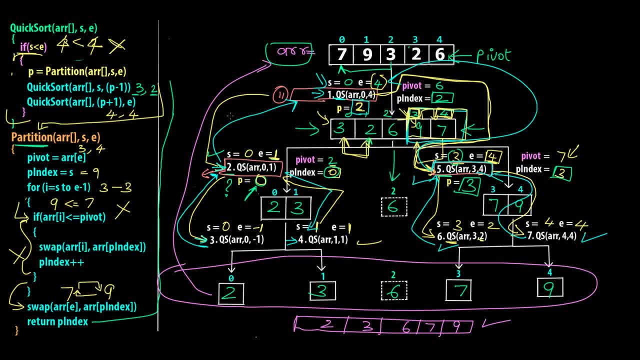 works. so, yeah, that's it for this video, guys, i hope you've understood the entire behind the scenes of the entire working. we've dry run each and every step and we've seen how the recursion progresses: how one quick sort calls and how one quick sort calls and how one quick sort calls and how one.